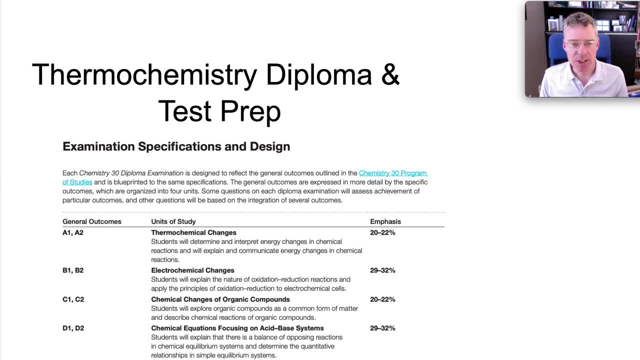 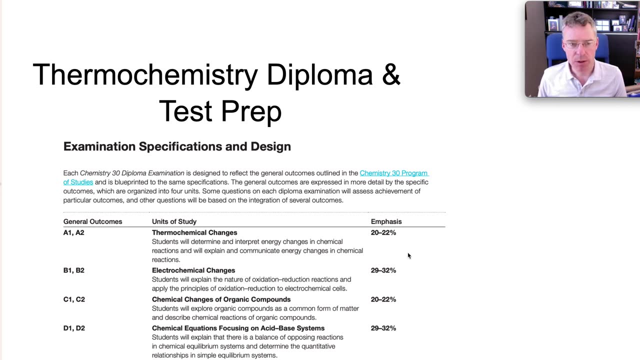 This video is a thermochemistry diploma or test prep guide. The emphasis will be a bit more on preparing you for the diploma exam, but this works just as well for unit tests you might have in thermodynamics Specifically for the diploma, and that is for this year, 2022-2023,. but these 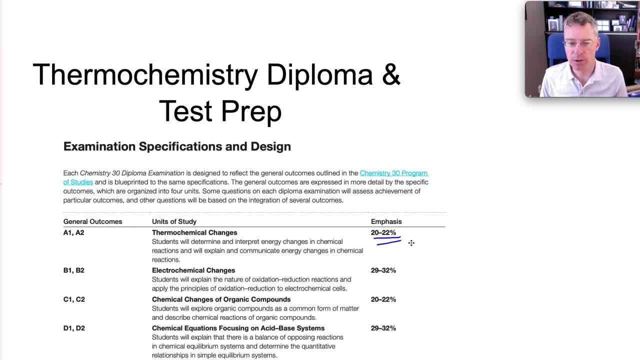 weightings never really change. Thermochem is going to be a little over 20%, so you've probably seen in your gradebook a similar weighting for this unit. Out of the 60 questions, that means you're going to get approximately 12 on thermochem. So the outcomes to 20 or so are going to have to. 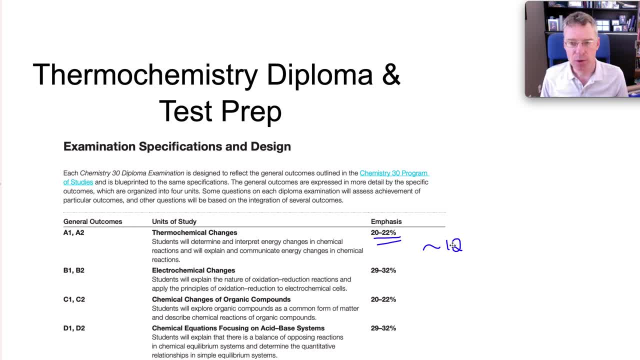 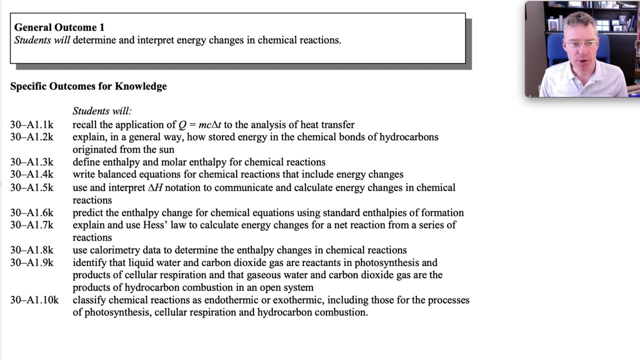 be sort of condensed into just 12 questions. There's about 12 because this is for multiple diplomas and you also have overlap between one question might have multiple units on it. So there's two general outcomes for thermochem. I'll go through sort of each of these outcomes and potential questions and using old 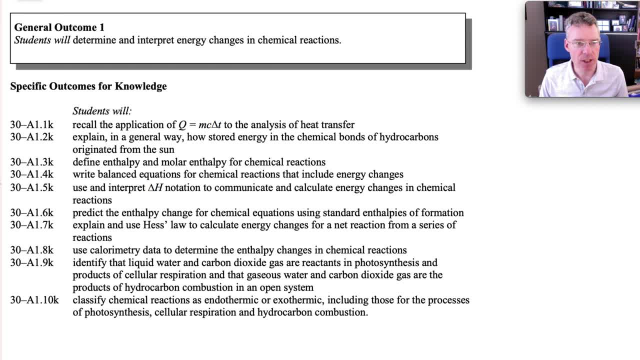 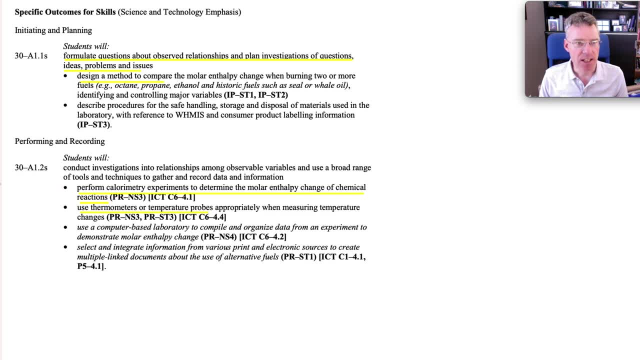 release diploma 2017 and 19 questions. The first one is around interpreting chemical reactions and the energy changes. The second outcome is about the graphical version. You also always have to be aware or have developed some lab-based skills, So, as a student, you should be able to formulate. 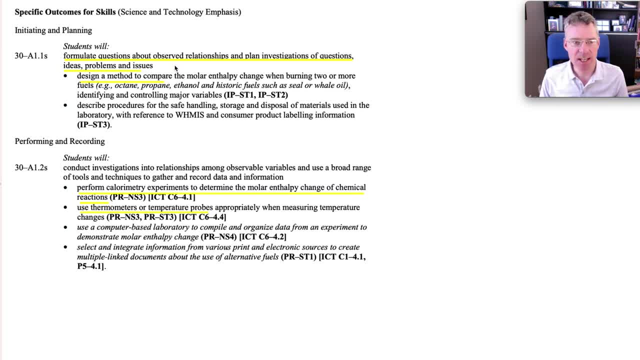 questions. You should be able to formulate questions. You should be able to formulate questions. design labs around thermochemistry particularly some overlap with organic chemistry is likely And you'll definitely be asked to not perform labs but analyze lab data. You'll always 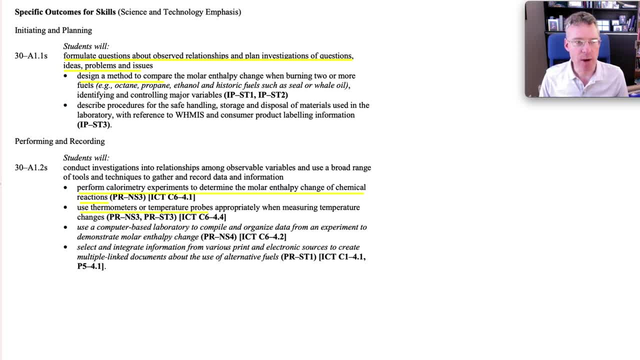 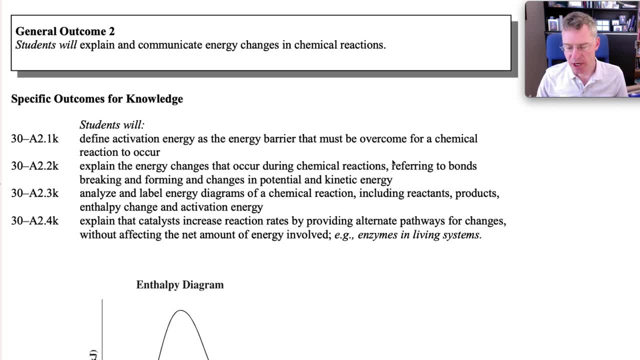 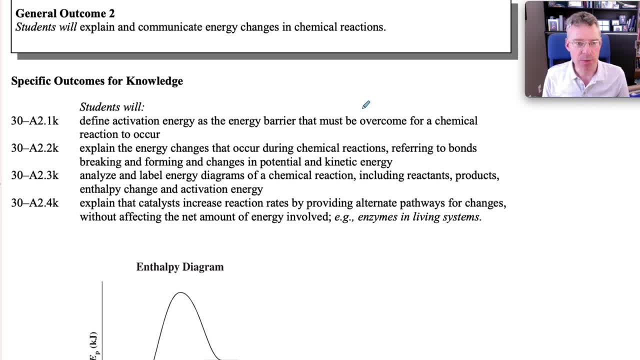 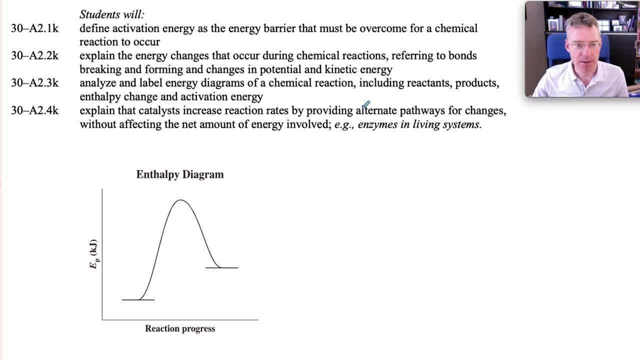 questions. You should be able to formulate the questions that you want to answer. So the other general outcome is that you're going to be having different daily served actions, so that's where you'll be having different reality bodies, And then, lastly, of course, um. 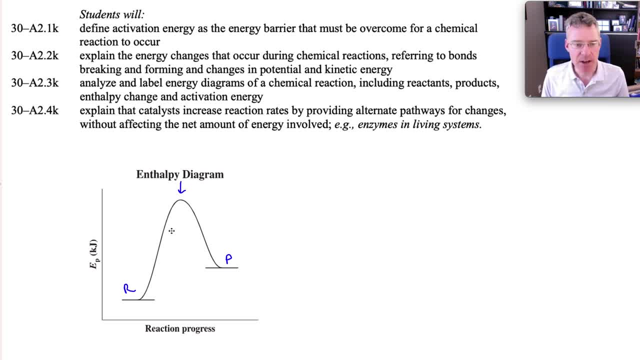 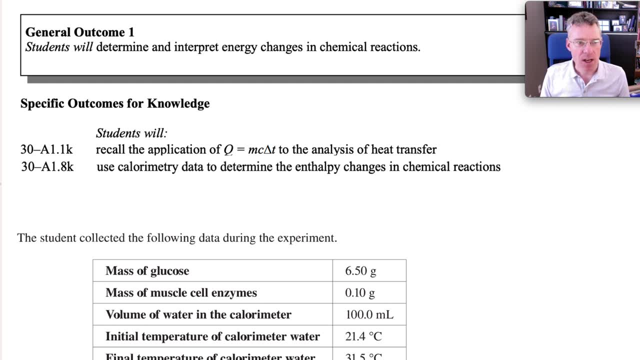 So you have your reactants. More attempts, more results. endo-exothermic type terms, So we'll get into those in the later part of this video. So, looking at some examples and details of the general outcome one, I've pulled two outcomes. 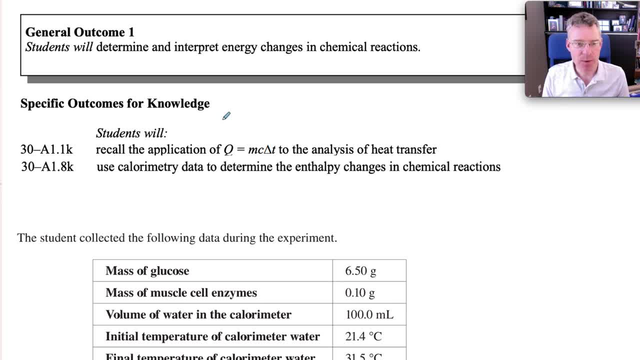 1.1 and 1.8.. You have to remember Q is empty, delta, T from science 10.. Most students have sort of forgotten that from grade 10, and you have to get a reminder in chem 30.. And here's a. 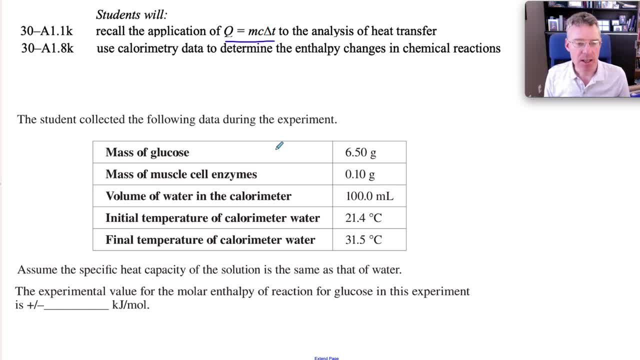 fairly typical thermochem experiment. Again, this is a question from one of the released items, So typical on an exam. you get the actual question at the bottom, So don't read through all the details. What is the experimental molar enthalpy of reaction for glucose? You need that. 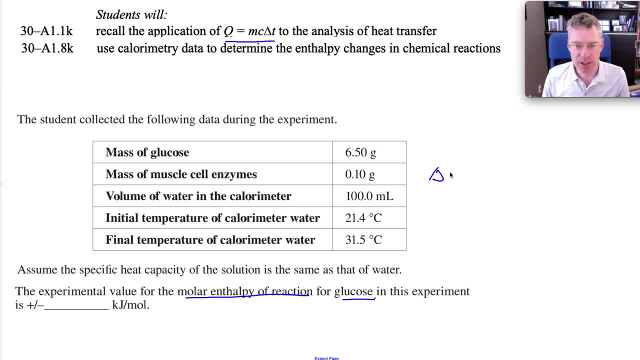 chemical. So we're going to need the change in enthalpy and we're going to need the amount of moles that released that energy, And that's why paying attention to chemical is sometimes very crucial. in this case, There's sort of really just one mentioned. You just have to realize that this enzyme is not something that. 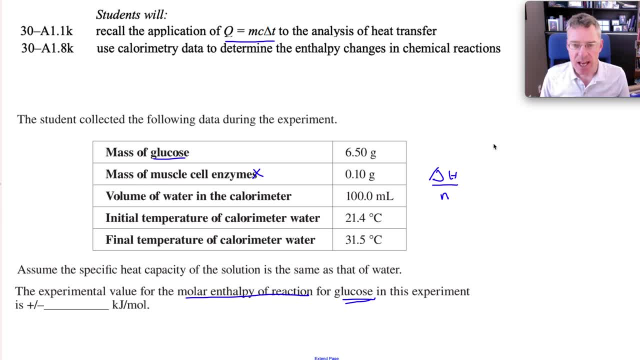 reacted So you can get enthalpy change from Q is MC, delta T. Again, calorimetry will be on every diploma. Sometimes the energy that's released or absorbed will just go into water and sometimes into a water and a can in a combustion reaction. If you're whatever surrounding details you're 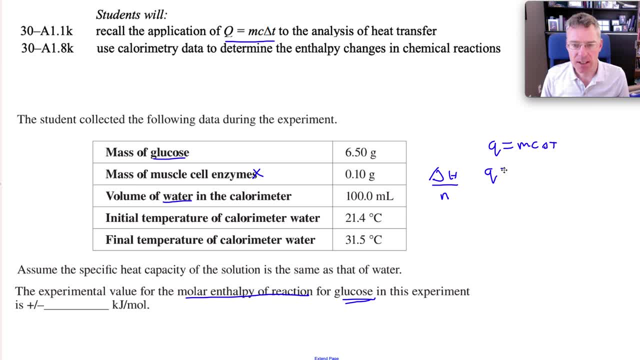 given you must use. So Q in this case is a hundred point zero. milliliters would be equivalent to grams. This is going into water. It's very common on diplomas now to have a non water surroundings to make sure students just don't always use four point one, nine joules per gram per degree. 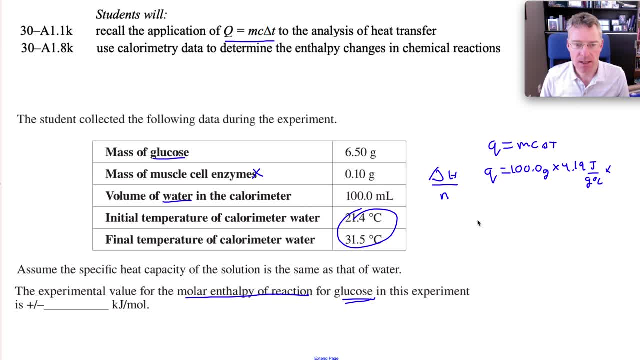 Celsius and your delta T is ten point one, So that gives you the heat or the Q, and I got four hundred and 4232 joules, or four point two, three, two kilojoules, So that gives us our data. we need to get our enthalpy change. we've got our energy and this is 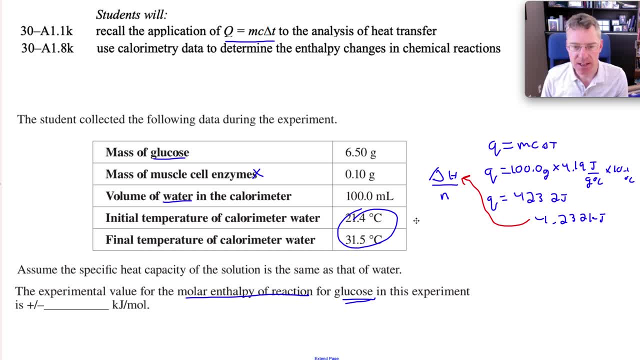 a warming up, the final temperature is hotter, so would have a negative enthalpy change. then we just need our moles, and the only thing really to watch out in this question is making sure you're just using glucose as mass, not a catalyst. an enzyme would be a catalyst that's not used. it's not what's reacting, don't. 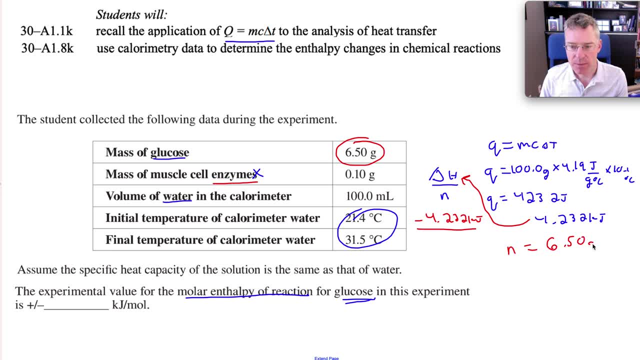 include it. so we've six and a half grams. I'm doing mass over molar mass and the molar mass is a hundred and eighty point one, six, I believe, grams per mole. so this comes out to 36, a little over 36 millimoles, and you end up with a molar enthalpy of negative. 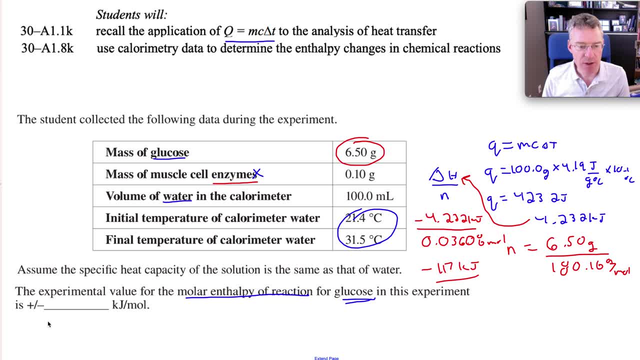 117 kilojoules. now, in this question, whenever you see this plus minus on a test or diploma, you're not keying in that, you just be keying in one one: seven, seven, as your answer to three significant figures is the delimiting amount, the 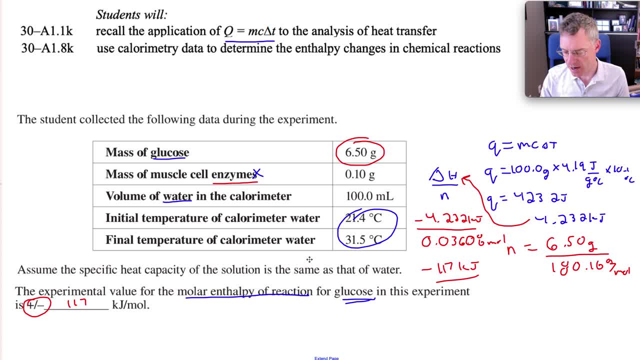 diplomas always tell you how many significant figures. I just cut it off this graphic, so hopefully this was a fairly straightforward MC Delta T type of question. I won't do any math with the surroundings, with two surroundings, but I'll talk about it in a later question, so definitely expect calorimetry. that's. 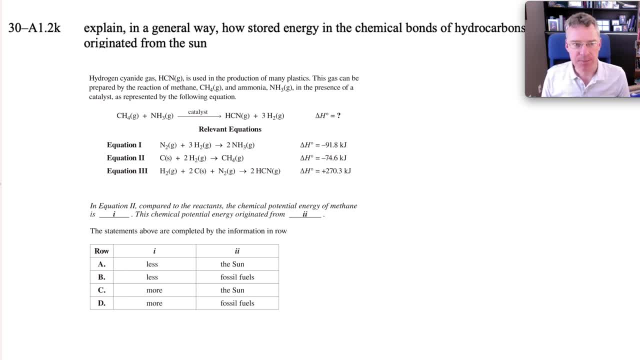 one of the twelve. there is kind of this annoying outcome that you need to know that energy started. hydrocarbons ultimately came from the Sun to anything seen age only reading through the question is only going to distract you. this is sort of a- I thought more of a confusing one in equation number two. so 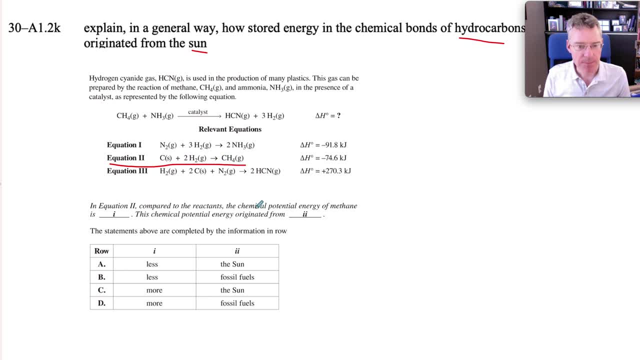 that is this one, the talks about the potential energy difference. I don't want to address that, but the potential energy originally came from it's a hydrocarbon. don't look at the energy which we just talk about, but the potential energy came from if it's a hydrocarbon. don't look at the energy, the energy that you would be capricious. but the energy that you would be capricious, originally it's a, which is a very Chinese word, but the energy and thePP, the energy we're talking about, is a question which we're not talking about is essentially nothing. but you know there, if you think that it's+, how many zero cubic meters per hour. it's 20 pi by 90Rep Payment. oh, you know, there's about 30999. 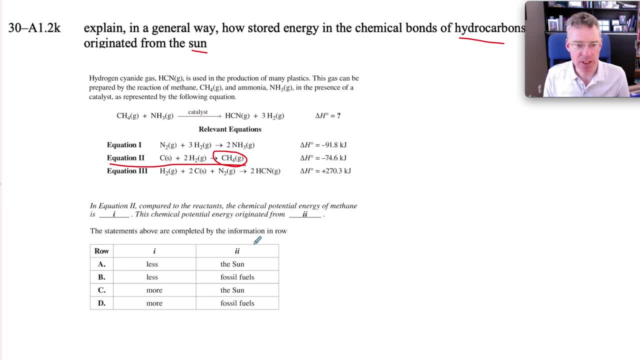 energy. don't try to do Hess here. that can really confuse you. this is a hydrocarbon and you need to know that all hydrocarbons ultimately had the energy come from the sun. okay, and then you just need to deal with the other part of this question. there was a time where we'd have questions that 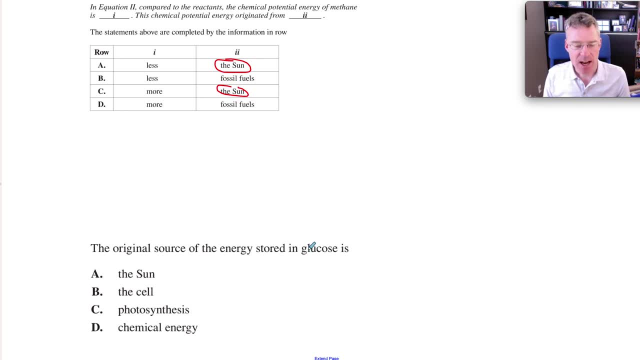 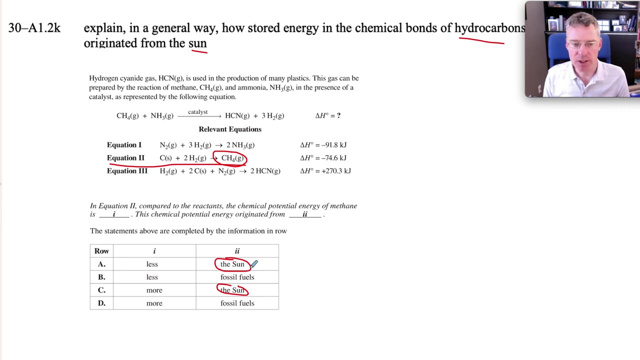 just talked about the energy in some sort of hydrocarbon, or in this case glucose, which isn't actually a hydrocarbon but it's close a derivative. but that still came from the sun and photosynthesis. so no longer are the questions sort of this easy where it's direct. typical diploma questions one. 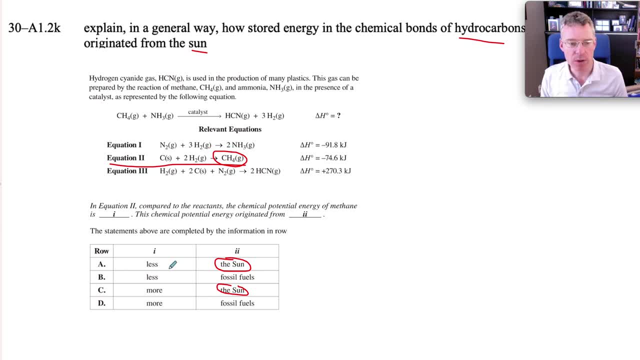 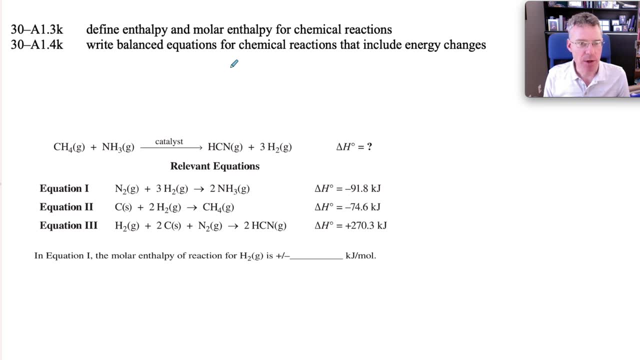 part is the sun and one part relates to endo or exo or potential or kinetic. so circle the sun. that's again always a small question. there's a couple outcomes around enthalpy, molar enthalpy and in equations. students often overthink these and they they make them more difficult. 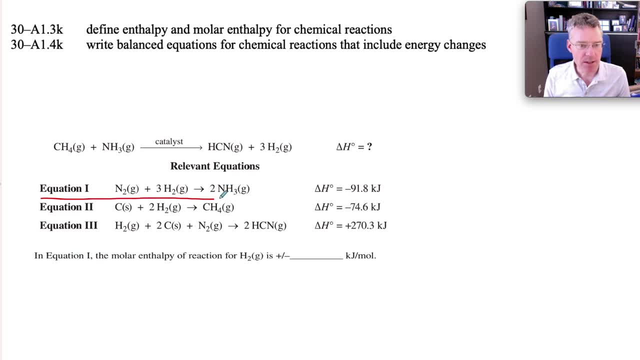 in equations number one, so we don't need to look at all the data in this question. what is the molar enthalpy of reaction? so all we need to do is set up a ratio. we need to find a enthalpy change and a corresponding moles, and we need to do this for hydrogen. so we got equation number one. 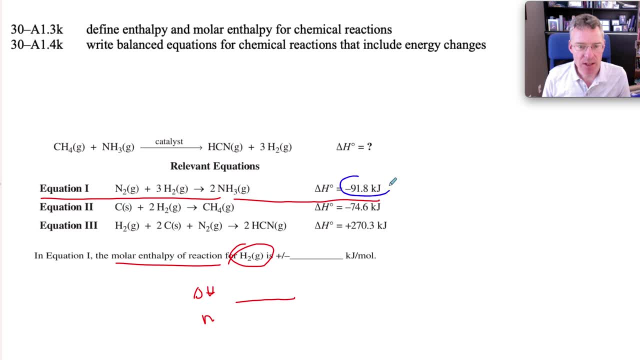 we know the enthalpy change change and we want this for hydrogen and there's three moles, so it's simply taking the 91.8 kilojoules and dividing it by three moles of hydrogen- no formation values, no need to look anything up, so you're going to get a value of a little over 30 or minus 30 kilojoules per mole. 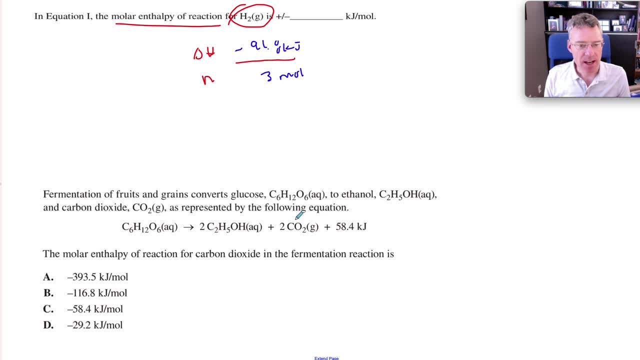 so expect this. it's on every diploma. another example of this below. but it's the same time that goes. it's going to change even more every time that. and you can do this with a Wolfram over-the-c? 민 type of thing. You just have to pull the energy term out. What's the molar enthalpy reaction for? 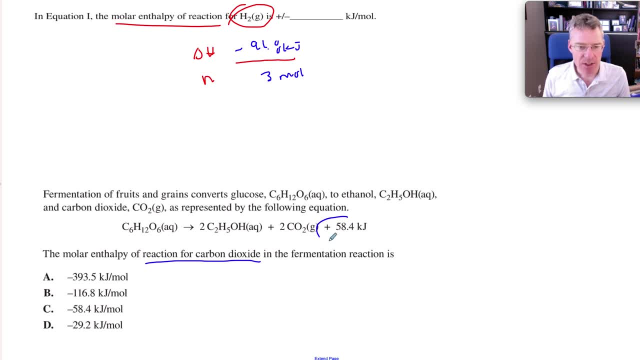 carbon dioxide. So we've got the energy. I just realized this is a product, It's exothermic. So this would have a negative energy, molar enthalpy, which all our answers are negative, And we have to divide it by, let's see, carbon dioxide, So two moles, So it looks like it's going to be D. 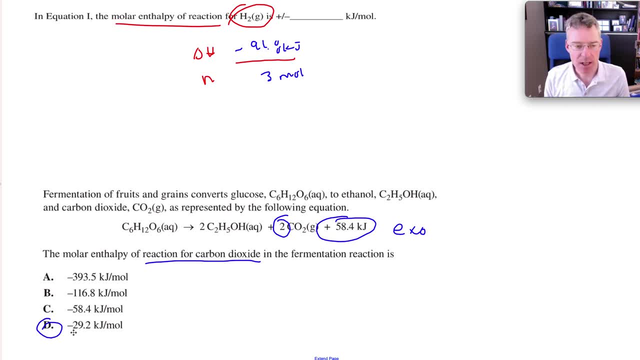 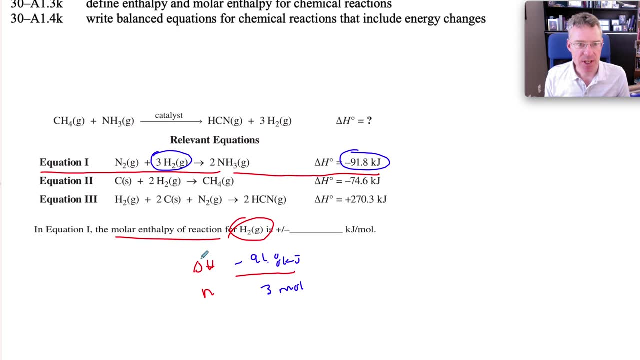 You often don't even need calculators for solving lots of these, So expect a pretty straightforward. do you understand what molar enthalpy is And can you pull it from some data? In theory, they could have given you a graphical version, a chemical potential energy diagram. 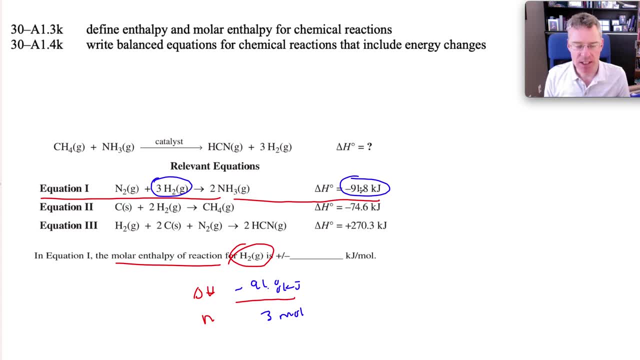 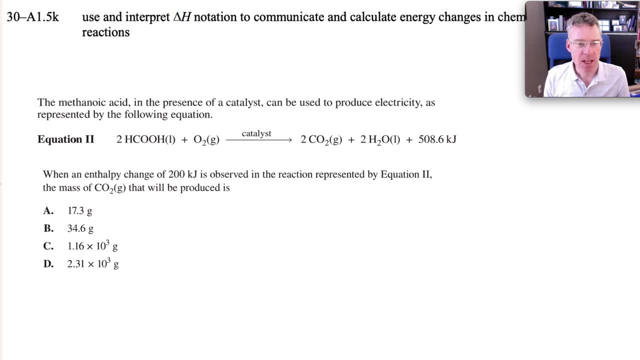 instead of an equation. It shouldn't matter Energy as a term outside the equation, energy in an equation graph. Don't overthink these. The fifth outcome: use and interpret delta H Notation to communicate energy changes. These are sort of using an equation or some circumstance. 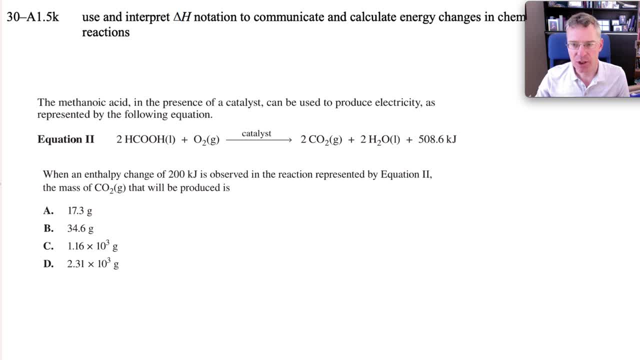 to answer a different circumstance, typically burning a certain amount of chemical. Now I solved these slightly different and it will work well. for this example, Instead of ever using molar enthalpy, I always tell my students change in enthalpy over moles for any one. 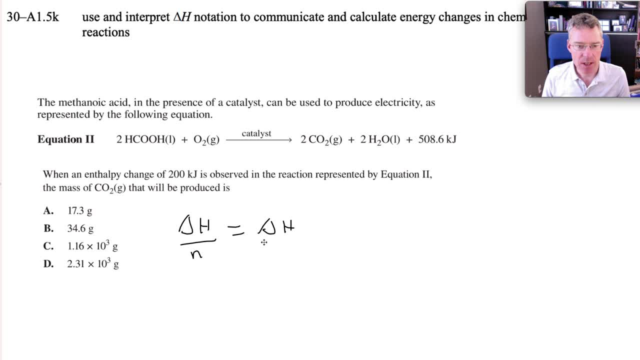 circumstance will equal the change in enthalpy Over moles for another. So you could use your equation data to fill in one ratio and then you could solve this ratio. if you're told you burned 10 grams or 100 joules or released, This question is a little different. 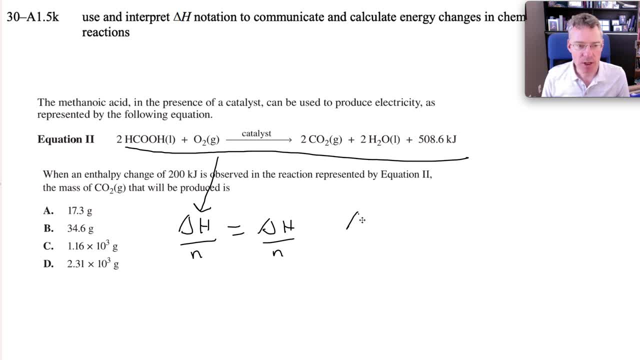 but the strategy will still work. This ratio will still work. for this question: What is the enthalpy change of 200 kilojoules? So something different from this equation. So we have 200 kilojoules released and we want to know what mass of CO2.. 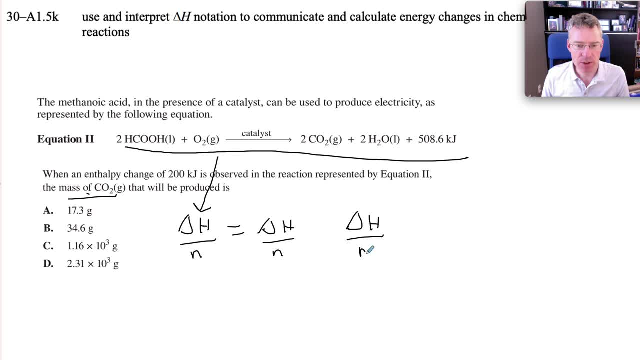 So it's not moles. they switched it to mass, But this ratio is still going to work: Mass to moles for the same chemical. It's going to be directly proportional. If you double the moles, you double the mass. 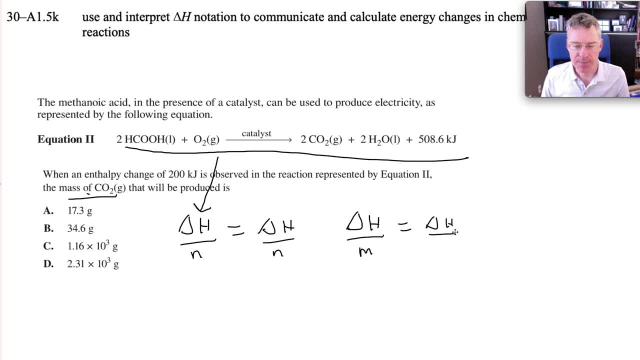 So if you double the energy, you'll need double the mass to also do that. So change in enthalpy divided by mass will equal change in enthalpy divided by mass, by mass. So in this question, using sort of our given information, we have a release of 508.6. 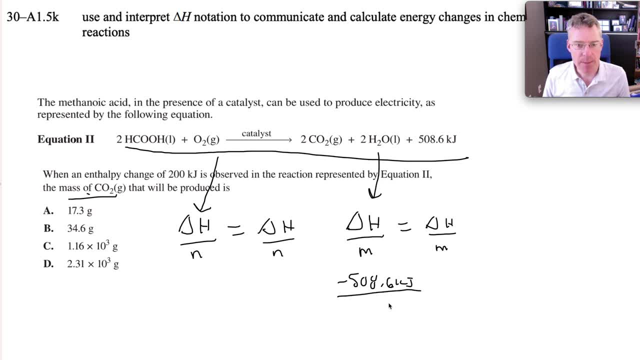 kilojoules for some mass. Let's see. this question talks about CO2, and there's two CO2s, So you need to know all how heavy is two carbon monoxides? So the molar mass is about 40, I believe. 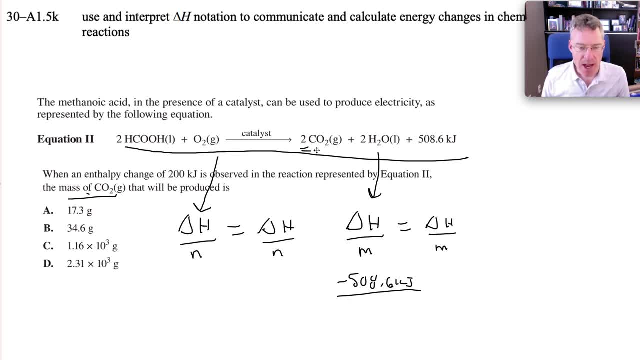 a little 44. So the mass of two CO2s is 88.02 grams. So again got the molar mass for CO2, and there's two of them. So that tells me you need to know all how heavy is two carbon monoxides. So the molar mass is about 40, I believe. 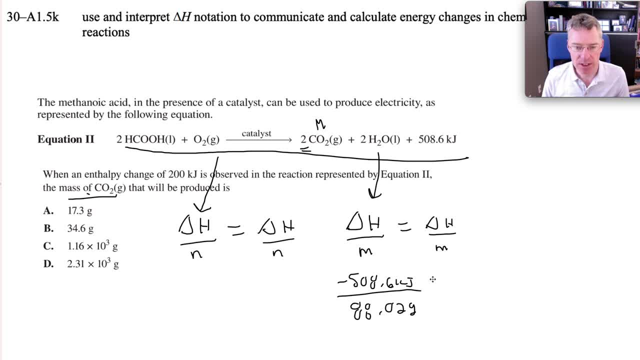 there's 88 grams needed here for the 506 kilojoules. And then we want to solve what if 200 kilojoules is released? How heavy would that need to be? And you can solve for this. When you cross multiply, solve for that question mark, you get 34.6 grams. 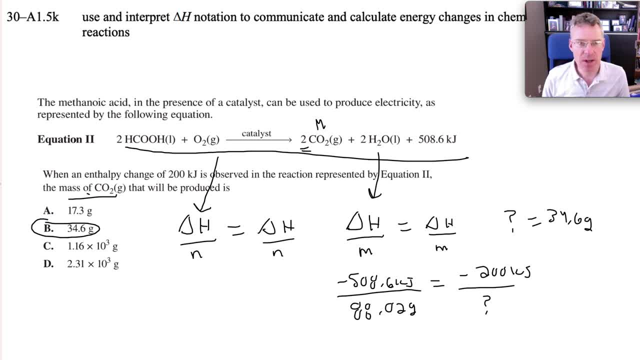 So this is a bit of a unique question, but what would be very typical you would expect in all diplomas is something like this, where it's just done in moles. This question tells you, or asks you, how many moles are expected of CO2.. And if this question 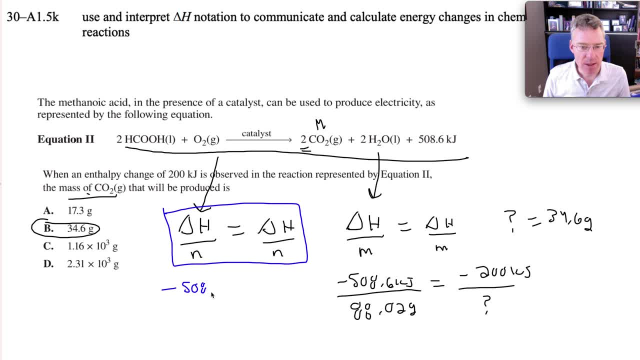 was moles, it'd be 508.6 kilojoules for two moles. It's not a bad idea to stick in the chemical. just to remind you, Equals okay 200 kilojoules When you cross multiply. you'd just have to replace that with the number of moles that. 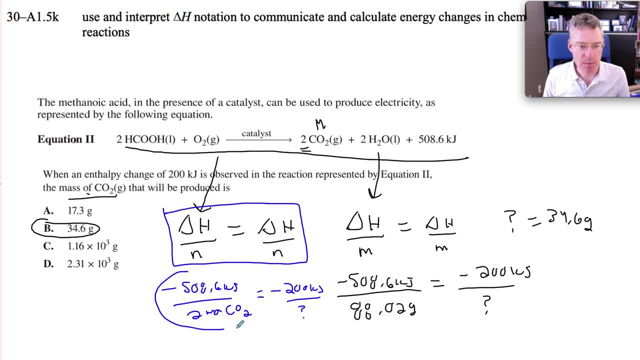 you've released or question mark moles, And this method would work too for this question: solve for the moles, and then you just have to turn it into mass either way, So expect some sort of question like this: This is just molar enthalpy and lets you solve a certain. 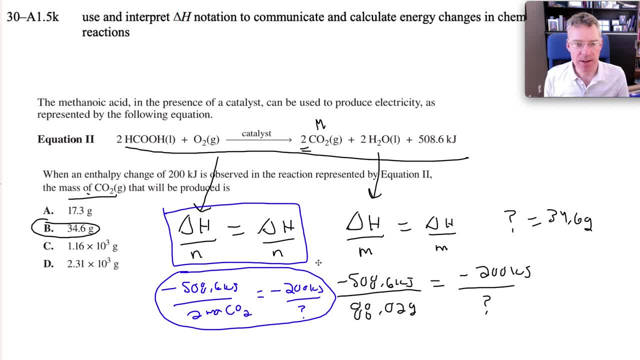 situation. So we know there's going to be a question about the sun, We know there's a calorimetry question or two. We know there's going to be a simple just what's the molar enthalpy for some data? And you'll definitely have some sort of question about the CO2 values And so 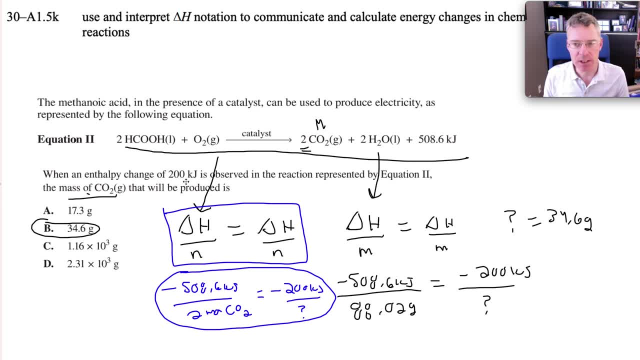 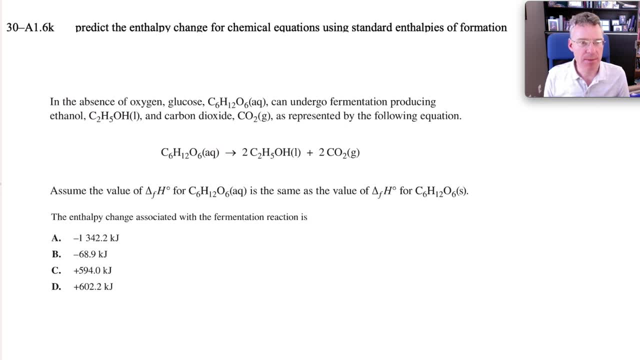 of question of what is the energy or moles released in in a different circumstance and you'll compare it back to an equation. so we're well over halfway through general outcome one. we're into sort of hessus law type of questions and using formation values predict the enthalpy. 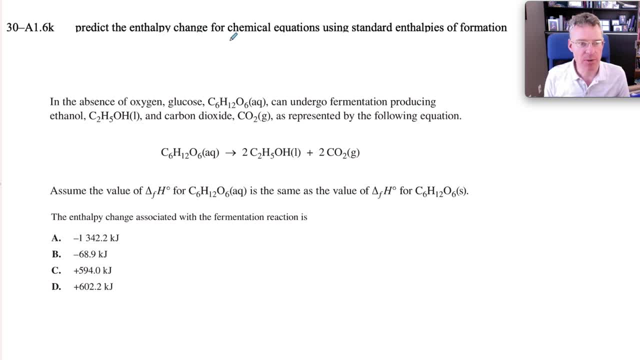 change for chemical reactions using standard enthalpies of formation. so these questions should stick at a. they'll talk, they'll um. they'll typically have no numbers given. if we look at this question outside of the answer, there's no values given. so you've got a. you know it's a hint. 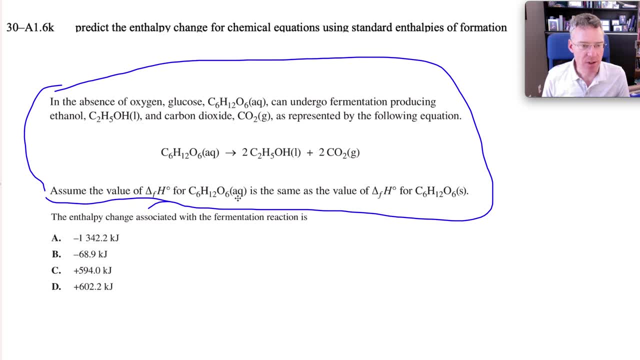 you got to go to your data booklet and use the formations and then you know, uh, implicitly they're talking about formation values. so you're gonna have to look up the products so to predict the enthalpy change you've got to sum up, so i'm just using a sum symbol of the moles times. 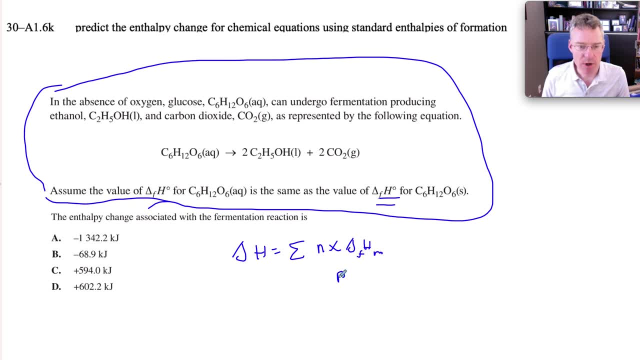 the change in molar enthalpy of formation of the products. so two times co2 plus two times ethanol and you're going to subtract that from the moles times the formation value you look up in your booklet for the reactants. so i'm not going to bother doing the math. 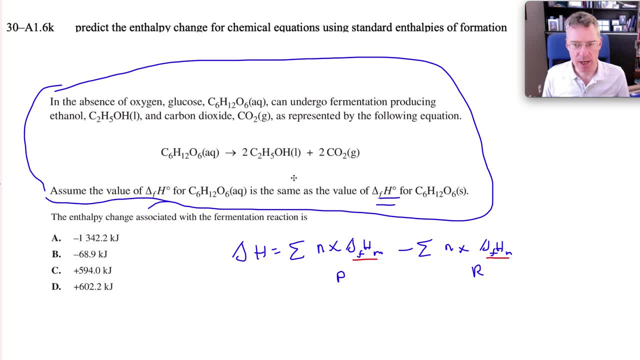 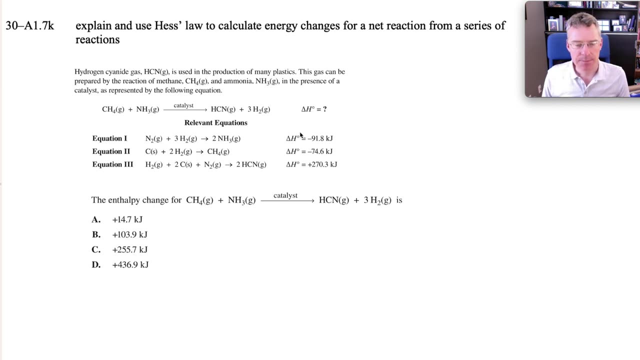 hopefully you've done this a lot in class and that's all this question is, and you should be expecting something like this. this would be a very straightforward one. again, this is a released item from an old diploma. you'll definitely get a hessus law question. i'm going to go through more. 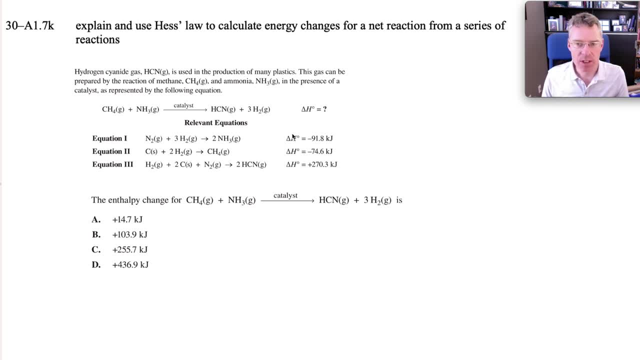 of a shortcut strategy for doing these when you notice that you need to use all the equations. you don't really have to write everything out. you can just figure what's the stoichiometric amount you need of each of the key chemicals and and sort of. do the math right away and not write and net and cancel everything out. 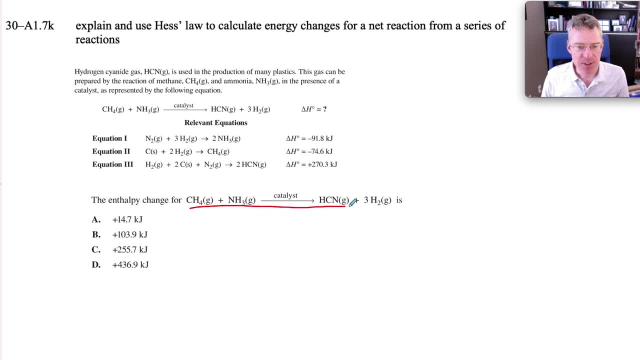 so we're asked to generate this equation and the first thing i want to notice is: do i have any extra data? and we don't. here we need to get methane, so we kind of get methane from equation two. we need to get ammonia. that's going to come from equation one, hydrogen sine. 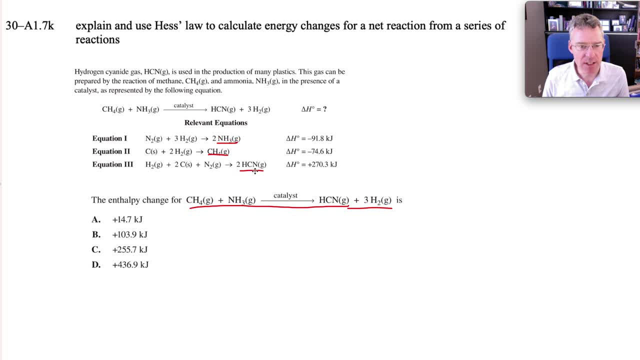 is going to come from equation three, so it looks like we need all of these and we're going to have to get the hydrogen to work out, but it's key that we don't have to get rid of any of these. so if i'm in a rush, i'm just going to figure out what i need to do to each of these. 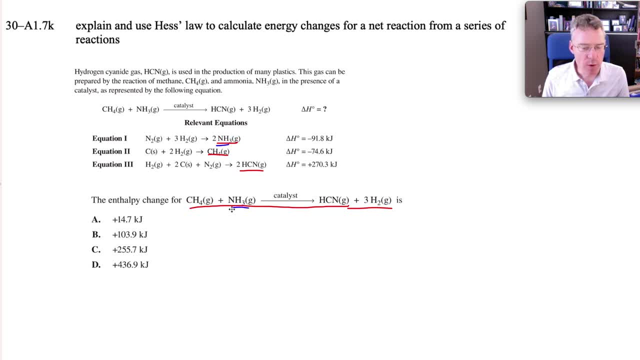 so if we start with ammonia, we want one of them on the reactant side and we've got two, so we're gonna have to flip this equation, which would flip this. and then we we have two of them, but we only want one, so we're gonna have to flip this. 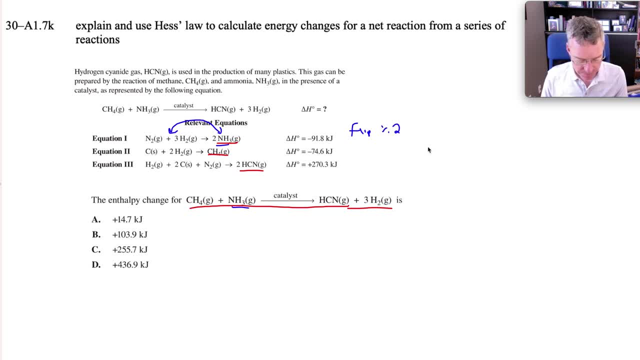 and we're gonna have to divide it by two. so if i flip that and divide it by two, you can sort of easily write that in your booklet you get plus 45.9 kilojoules. so it's just saving us time actually flipping it and writing everything out. 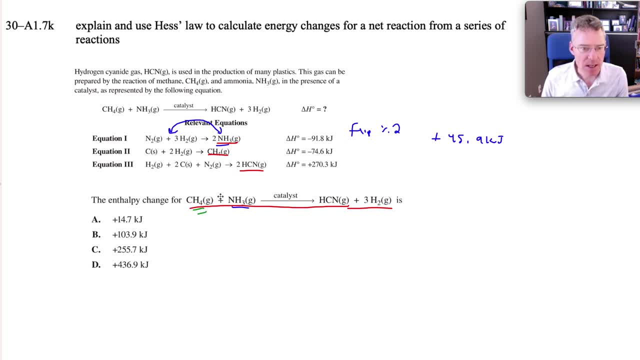 for methane, that is in the right amount, but it's on the wrong side. we've gotta, you know, flip that. so when we flip this one and the number stays the same, it just becomes positive 74.6 kilojoules. so that's going to get us these chemicals on the right side, or the correct side, which is the 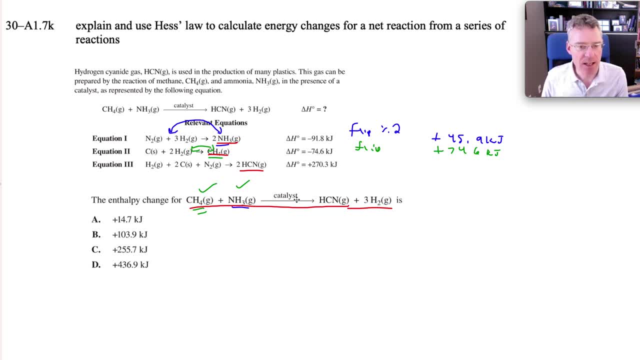 reactant side, technically the left side. last, we need to get our protein in thisEND💞 Doctor product. we need just one hydrogen cyanide. this has two, so you don't need to flip this one, we just need to divide it by two and we get our third positive value. you really got to watch your signs. 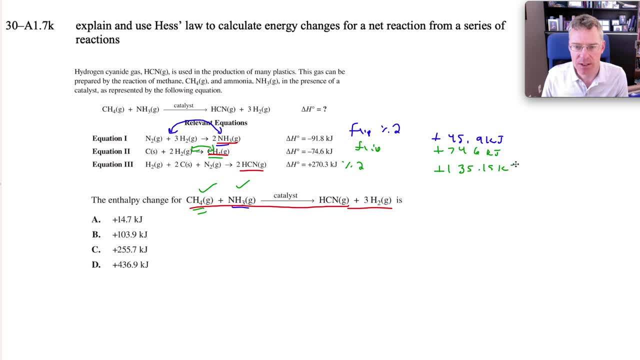 I definitely encourage you to always write in the positives and don't leave them out. so we can just add these all up. so these two are about 200 plus another 45- 50, so about 250. so you don't even need your calculator after doing those subtractions, the answer is going to come out to c. so if you're 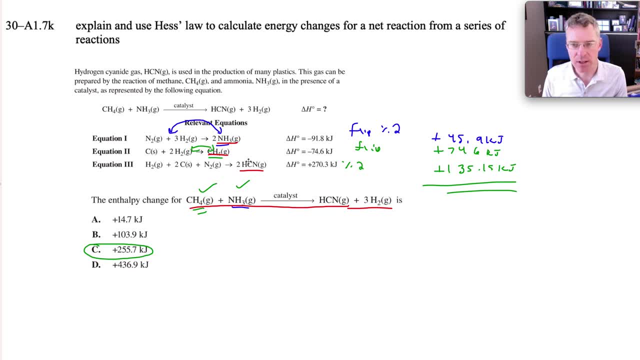 trying to save some time on Hess's law, and you know you don't have an extra one. you can just sort of do this. if you've got an extra equation, well then you may want to write everything out. it's going to take a bunch of time, but you will get to the correct answer if you're careful. 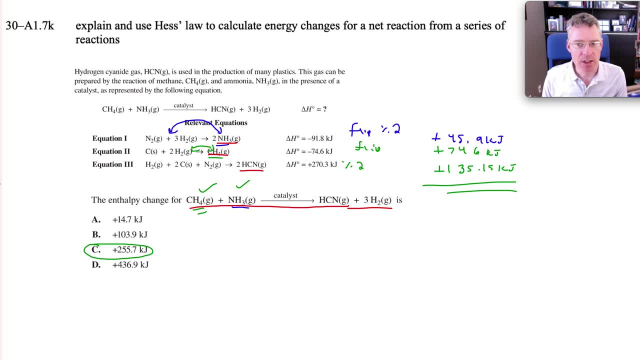 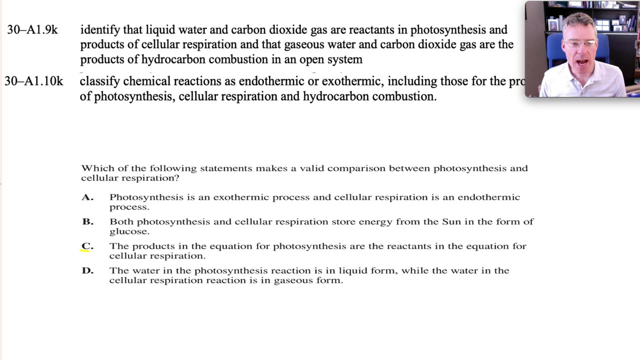 so definitely you're going to have a Hess question. so we're pretty much up to six or seven sort of guaranteed style of questions and you can hopefully practice this from the resources your teacher has given you. students often don't practice and teachers, including myself, don't spend a lot of time on emphasizing. you need to be familiar. photosynthesis cellular. 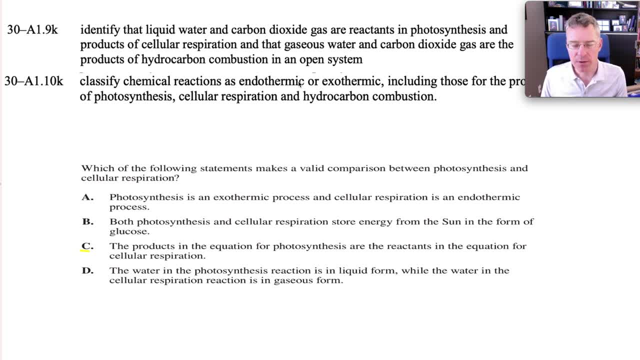 respiration when something is open versus closed. those concepts you need to be familiar with. photosynthesis, cellular respiration when something is open, sort of connect. so anything metabolic. so cellular respiration or photosynthesis, you're going to get liquid water. photosynthesis takes energy from the sun. it's an endothermic reaction, cellular. 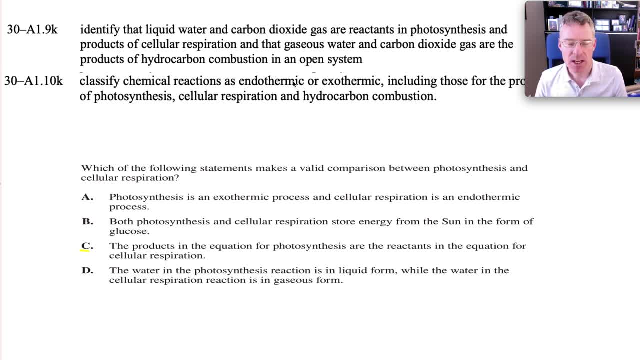 respiration is just like open combustion, except for it happens in a cell. so you get liquid water. open combustion, cellular respiration are both exothermic. you are going to get a question about these reactions that you understand: the open, closed and the state of the water. 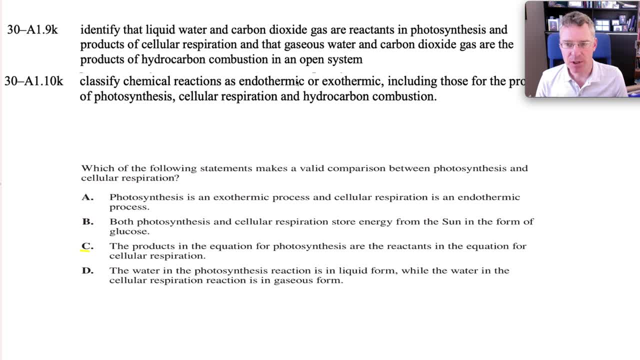 if you flip through a whole diploma, you often have the equations right in the booklet somewhere. you know, if you flip through a whole diploma, you often have the equations right in the booklet somewhere. so if you forgot something, flip through the whole exam and hopefully you'll get a bit of a hint or reminder. so this question from a released item: what's the phone statements? 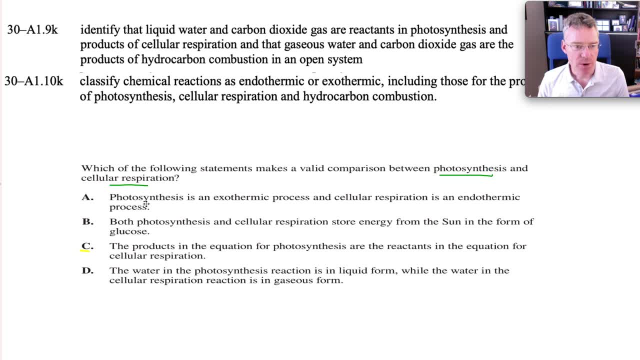 are valid between photosynthesis and cellular respiration. so photosynthesis is exothermic. no, it takes, it requires energy from the sun. it's an endothermic reaction. so we got a wrong statement right away. both photosynthesis andите look tremendous. that's it. you don't have to examine the results yet. 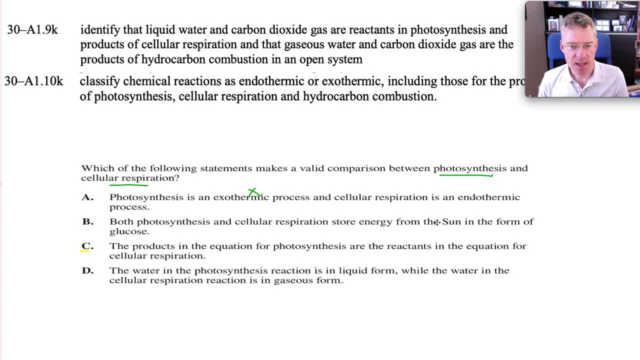 in cellular respiration store energy from the sun. No, photosynthesis does, Cellular respiration does not. The products in the equation for photosynthesis are the reactions in the equation for cellular respiration. That is correct. They are just, you know, the opposite reaction. 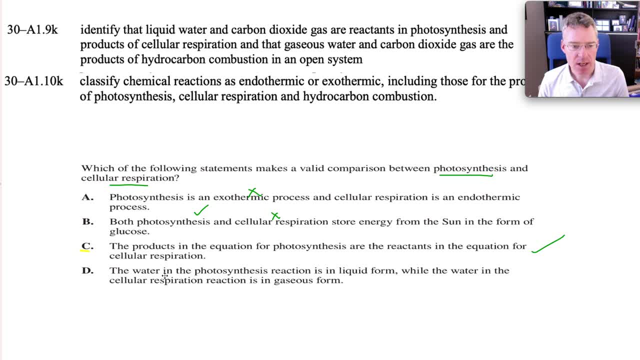 to each other. So that was the correct statement. Water in the photosynthesis reaction is in the liquid form. That's true, That's in a cell, While the water in cellular respiration is gaseous. no, it would also be in the liquid form. So lots of little true and false bits, but only C is. 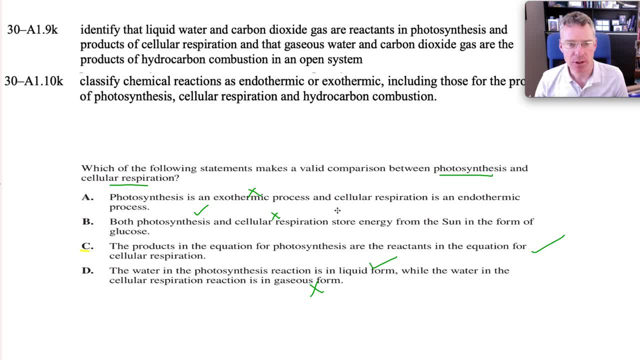 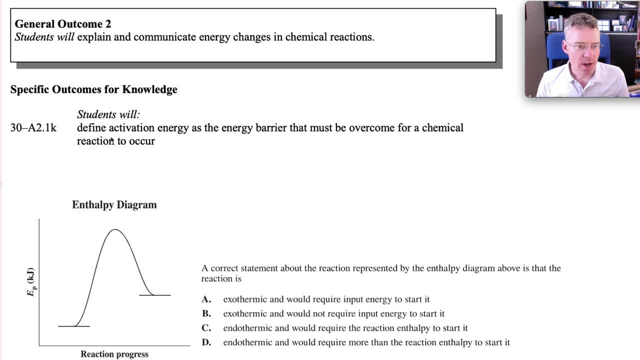 It's very graphical. So you have to be aware that activation energy is a barrier that's always there for all chemical reactions. So that barrier, if you look at your reactants, is up to the very top. This is your energy of activation. It has to be positive. It's always there. 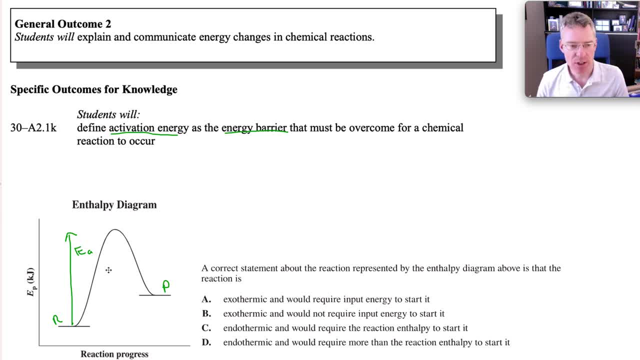 Even in an exothermic reaction it doesn't just happen on its own. Your wooden desks, if you have them, don't just burst into flames. You have to provide some heat or energy to get it started. So that would be the activation energy for the forward reaction. We'll talk about reverse. 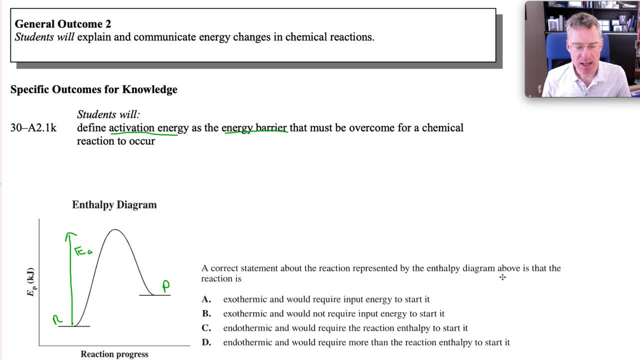 maybe shortly So- the correct statement from the following diagram that the diagram is exothermic and would require energy input to start it. This is an endothermic one. So those are out, And so it is endothermic and would require energy to start it. You always 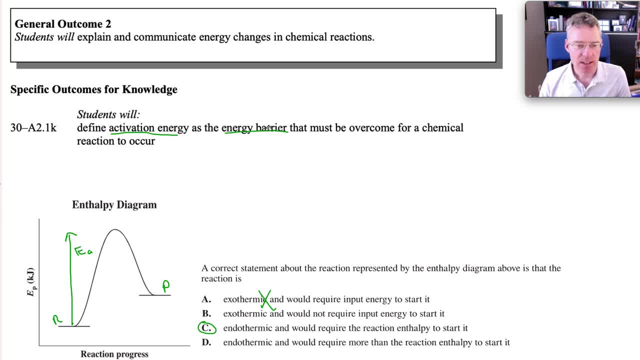 have to put energy in. So that's what this question is getting at. There is always a barrier, Don't think because something is exothermic, it just happens all on its own. So that's sort of the first outcome- activation energy- of the first specific outcome for outcome. 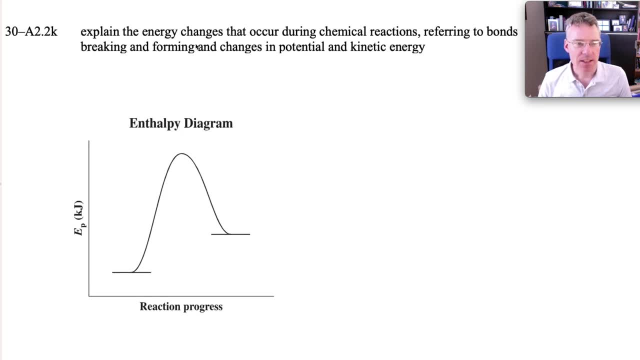 two. Second one explain that energy changes that occur in chemical reactions refer to bond breaking and forming. This doesn't typically go well. Students don't sort of fully connect the bond breaking and forming to these chemical potential energy diagrams. So we've got reactants, we've got. 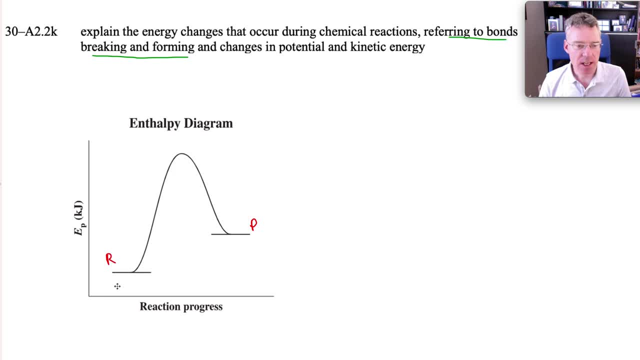 products. So the bond breaking is pulling things apart. Imagine you had hydrogen gas and iodine gas and you're going to react them and you got to pull them apart. The H's have to be separated, The I's have to be separated. This what we called activation energy before. but this going up is bond breaking. I'm 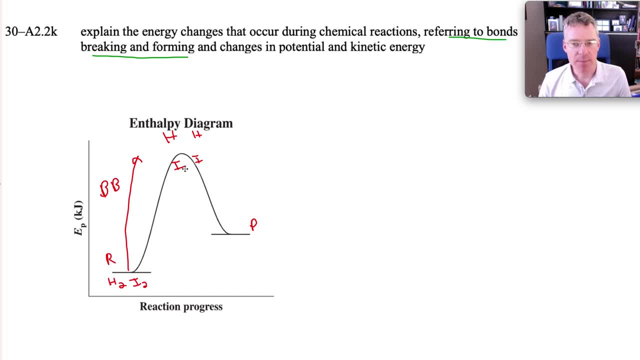 going to use BB for that. The first part, the going up, the activation energy is breaking bond. So the up is bond breaking. The down is when these are apart and they come back together in a new combination. So the down Is the bond forming. It's always like this: This is crazy, oversimplified Reactions don't often happen. 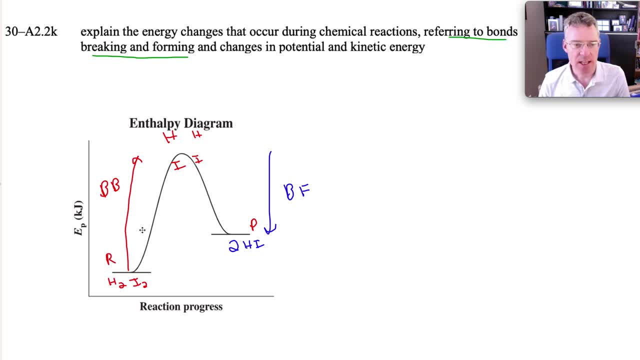 into sort of one step. But for chem30 they do. The up is the bond breaking, The down is bond forming. It's always energy being put in in the bond breaking and you always get energy coming out and the bond forming. In this particular example, this graph the energy that needs to be put in to break the 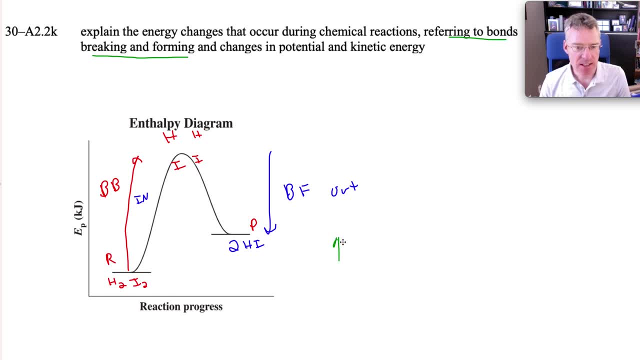 bonds is greater than the energy you get back. So net this is a endothermic reaction. where delta H is greater than zero, There's more potential energy. at the end We didn't get as much out. So bond breaking up, bond forming, coming down. 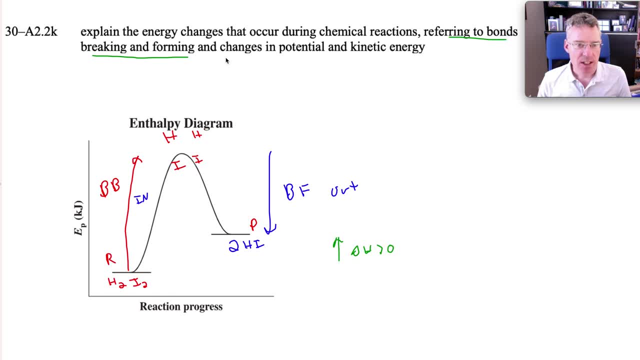 Um, the changes in potential and kinetic are kind of different. It's the same outcome but you have to kind of separate things. So this whole graph is potential energy. This is the difference. bond energy had to be put in to break the bonds. Potential energy: put in some potential. 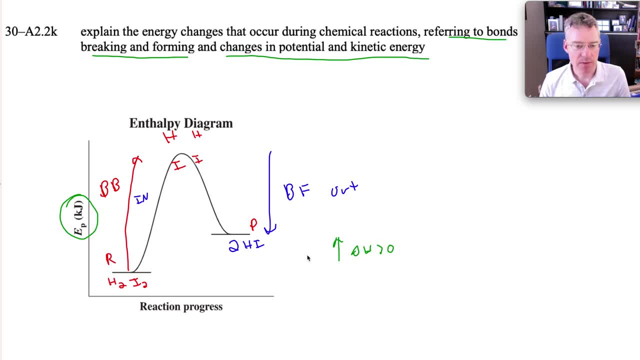 energy was released in the bond formings. We have a difference in potential energy, So I'm going to relabel this. Potential went up. We have the law of conservation of energy. So if you have more potential energy now, where did it come from? Well, it came from an equal decrease. 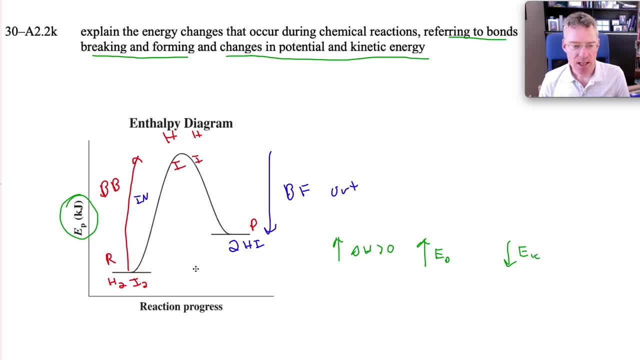 in energy kinetic. So we kind of talk about potential all the time in these graphs. That's the enthalpy change that you've talked about all through your course, but there's an equal and opposite kinetic energy change. Now this is what we actually measure. 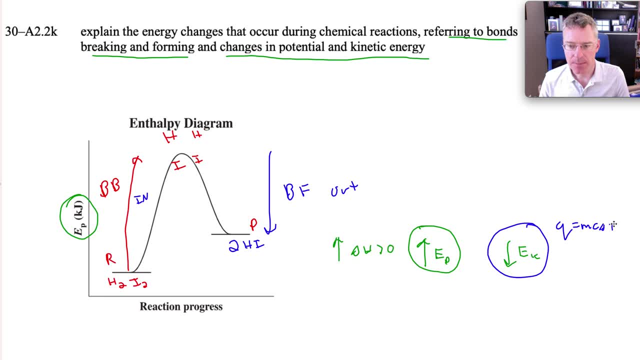 This is what we get when we do. q is mc, delta, t, And this gives us a number. Enthalpy, or q, is actually a scalar, not a vector. You shouldn't be putting a sign to it, but this will tell us how much kinetic energy difference there was. 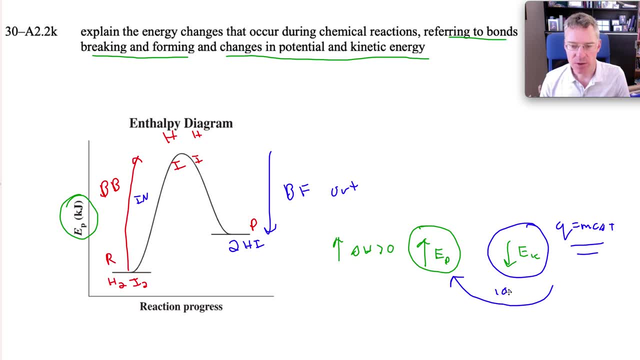 And we equate that back to potential And we just assume there's a hundred percent efficiency here. So if the water cools down, that means cool down, So it was endothermic, So that means there's an equal but opposite change in our 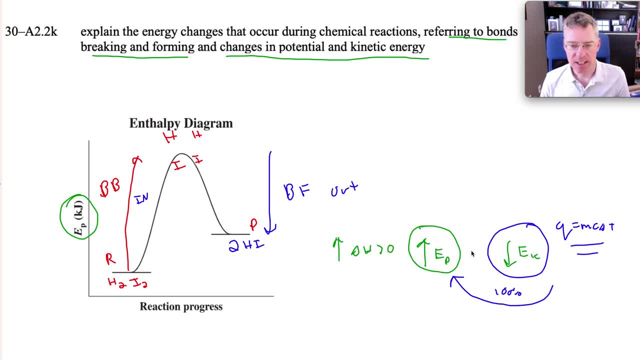 potential energy. So we got these sort of equal but opposite to each other, equal in magnitude. I'm just sticking absolute value symbols around it. A big thing to emphasize here is the bond breaking and forming. Hopefully this potential kinetic swap was an important part. 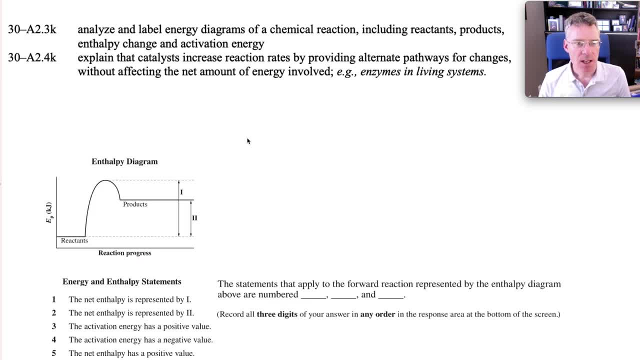 of the start of your unit. Last outcomes around catalysts and labeling. This diagram doesn't have a catalyst on it, But what catalysts do is just give you an alternate pathway. Don't worry about how enzymes work. That's way beyond the course. But no matter what catalyst you put in, it is going to create a. 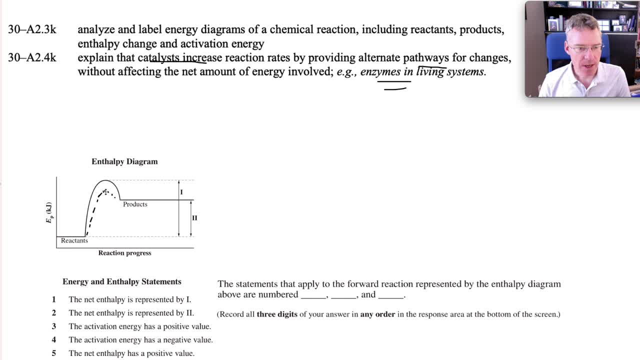 lower barrier. We know that the barrier is going to go above the products where you used to have an activation energy that was this high. So we're going to go above the products where you used to have an activation energy that was this high. We now have one that is shorter- Pardon my crooked line- And that's all you really need to know. what catalysts do is. 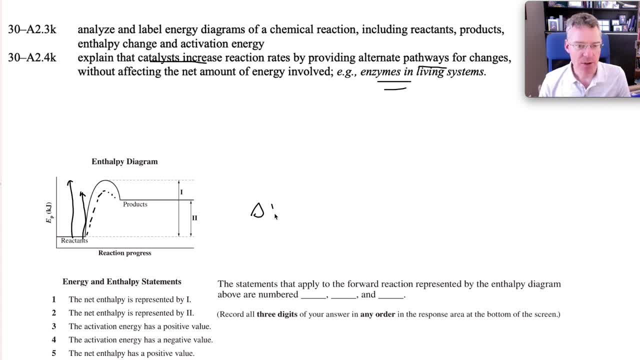 they drop that barrier. It's key that you know that the enthalpy change is the same with a catalyst. Why would you use a catalyst then? if the energy changes is identical, Well, you get there faster. So if you're going to release 100 kilojoules, it's going to take a minute. 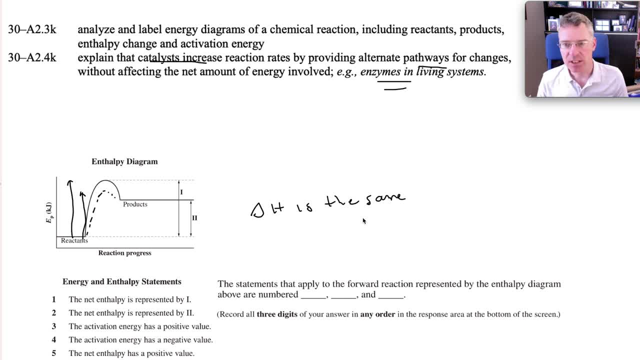 maybe you get that 100 kilojoule release in 15 seconds. often it can be orders of magnitude faster, but no change in delta h. now rate of reaction is not something studied in regular 30, so it's. it's just not a topic. you have a lot of experience with advanced placement. 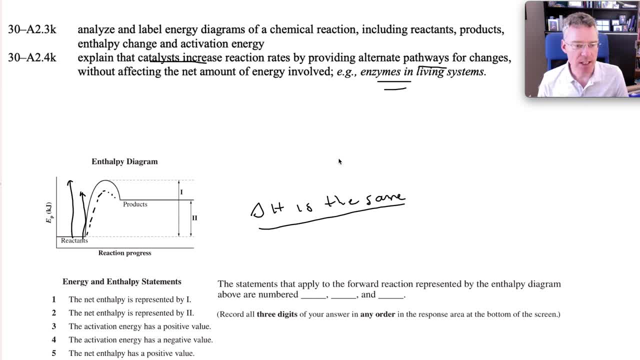 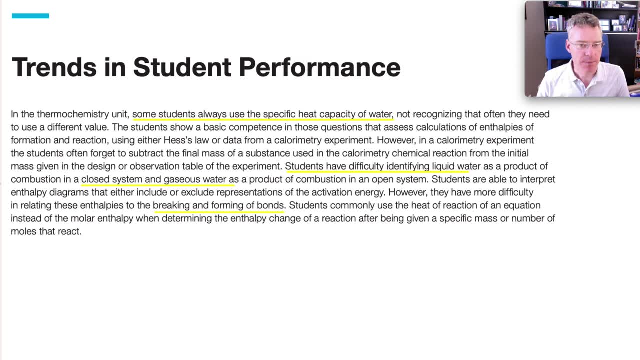 students would have spent a whole unit in high school on rates, but not most students last. the alberta ed bulletin for chemistry has some comments, uh, about trends in student performance and common errors, so i just want to highlight some of those fairly quickly and make sure that you are aware of these common errors and hopefully your teacher prepared you. 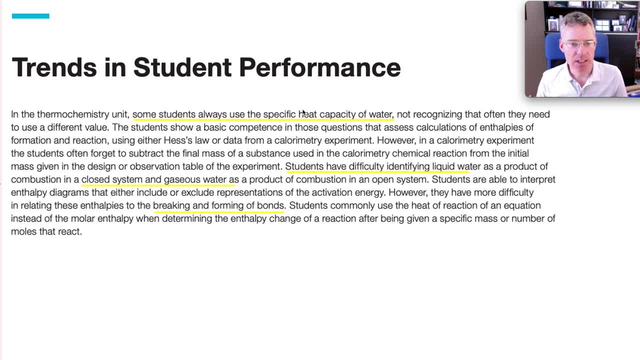 well, and you can sort of emphasize these pieces even more than your teacher might have in in a limited time. they probably might have done that in a limited time. so i just want to highlight that. you're right there. you're able to re-evaluate the performance of the tests. 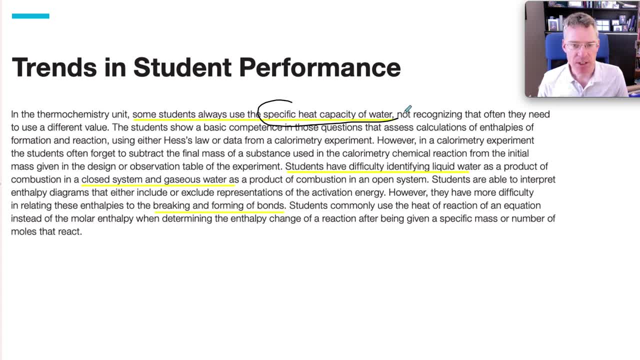 or even you know the level of learning that I have had to get through this unit. so there's a warning. some students just always use the specific heat capacity of water and most diplomas now will have a question where the heat goes into- maybe a block of aluminum or a block? 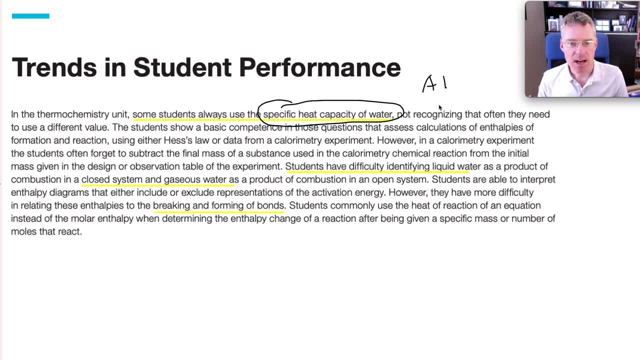 of iron. we definitely put this on our unit tests in my school. so make sure you're reading the question. if the energy isn't going into water and you have to do mc delta t, you look up on page three of your data booklet. there's iron, aluminum, tin. i know we're going to talk about the energy level. 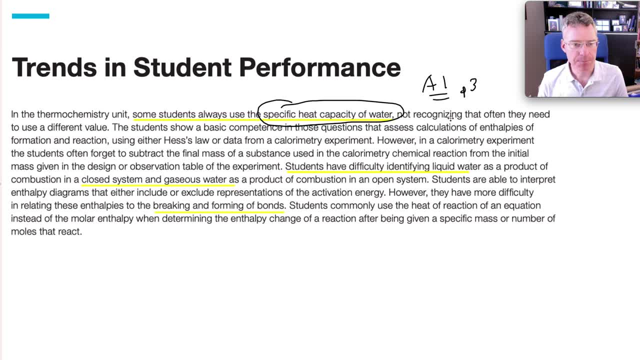 as well and you have to do mc delta t. you look up on page three of your data booklet. there's iron water and probably a couple others that they could ask. second comment they have, or that i'm highlighting, is just being aware of that liquid water we talked about. you need to be aware of. 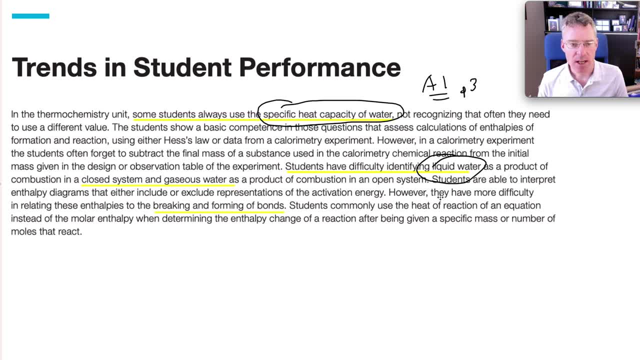 photosynthesis, cellular respiration. it is going to be a question. make sure you prepare for it. and then, last, i'll highlight this- bond breaking forming is a concern they have in the trends for student performance. so make sure you realize the bond breaking is the up part, exactly the same as 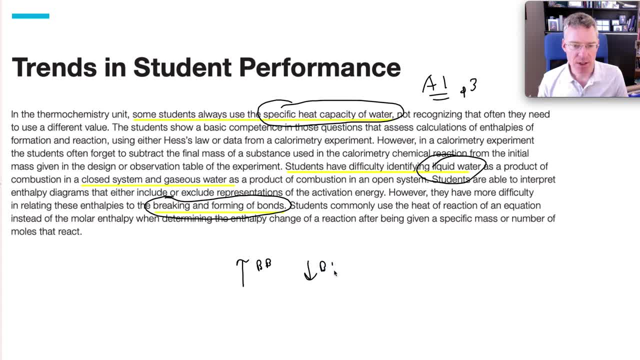 activation, energy. bond forming is the going down, the release. so in and out you always have to break bonds, first going up, and then you get new bonds formed. if you don't break bonds and form new ones, it's not a chemical reaction and that's not what we're and we're studying chemical reactions in. 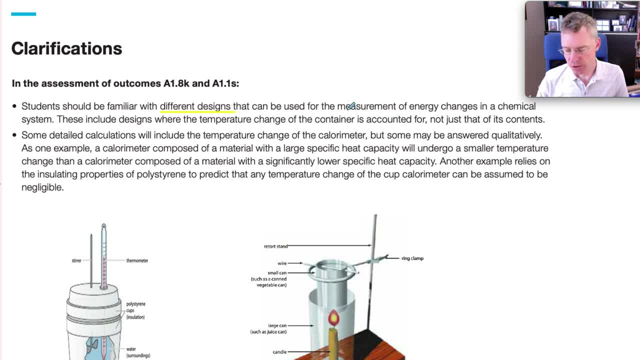 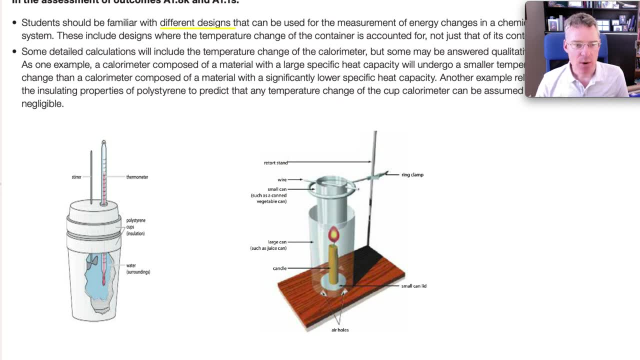 this unit. a few other specific details. students should definitely be familiar with multiple designs of calorimeters. back a decade ago i was a little guilty of just sort of focusing on your styrofoam cup calorimeters. where q is a lot simpler, it's just mc, delta, t of. 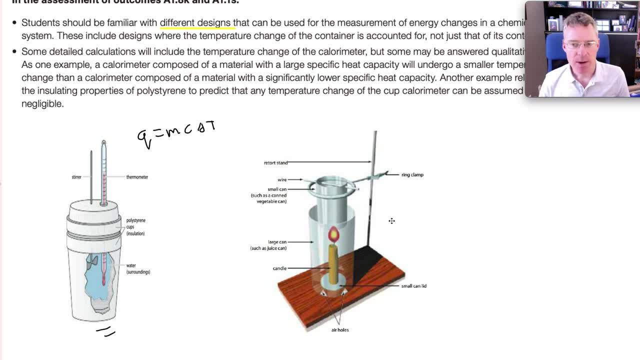 the water you could ignore. the styrofoam combustion shows up in diplomas almost all the time. there's so many design problems, efficiency problems of losing energy coming out the sides. but i want to particularly emphasize that you might have to do a q total with this design. you might have to do 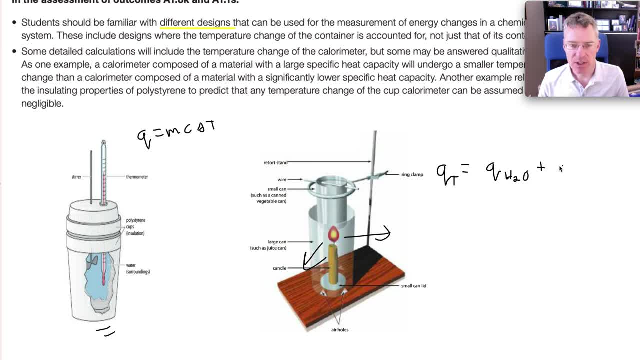 q of the water and if they give you the data for this metal can you'd have to include that? you know, often it's aluminum. in the labs we do in my school we just use aluminum cans and then students can weigh them and we're going to assume that the delta t of the water is the same as the delta t. 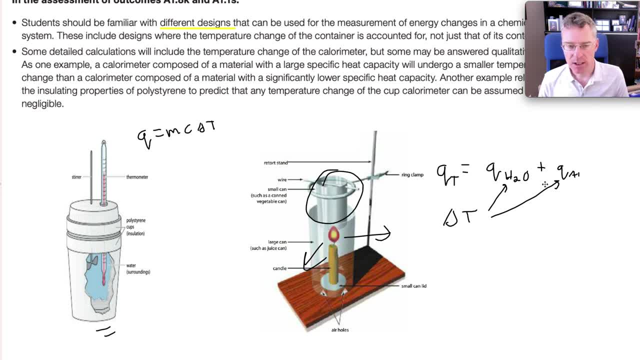 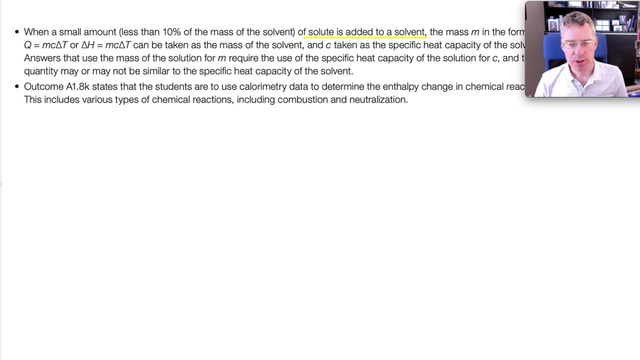 of the metal. if you let them equilibrate they should go to the same delta t. so two setups make sure you can do calorimetry experiments, uh, with both. one of the assumptions you have to make in calorimetry for solutions that are dilute is: 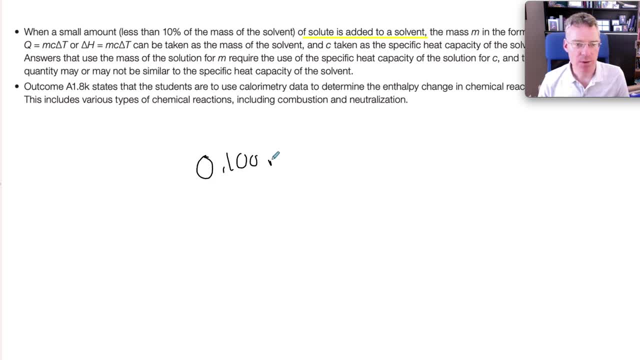 is just using the solvents. if you have 0.100 moles per liter of hcl, then you've got 27.5 mils of this. okay, uh, it's talking about using just the, the solvent for the solution. okay, so for for doing your calculations. so we'd assume this is mostly water, so pretty close to 27.5 grams. 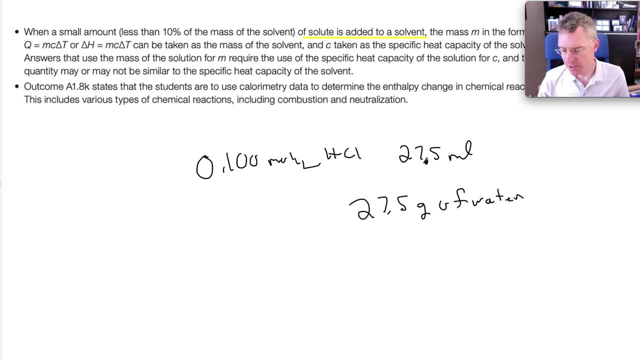 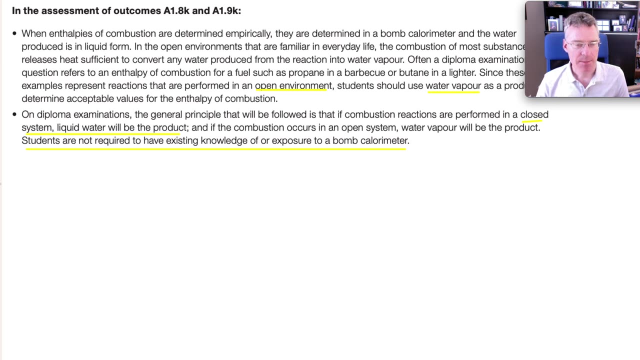 of water and you'd use the specific heat capacity of water. you've maybe been doing this and not even realizing you've been doing it with. with dilute aqueous solutions, everybody does an acid base neutralization in calorimetry, typically the start of a course um the common. again, i'm just 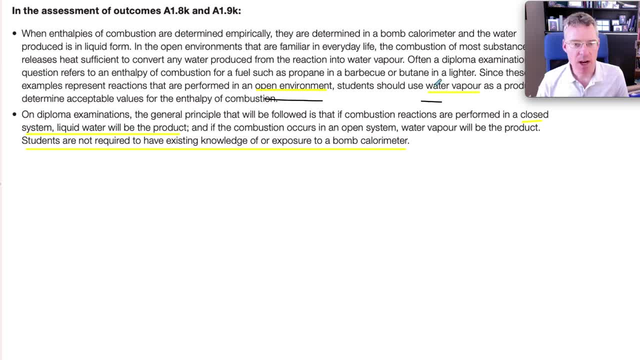 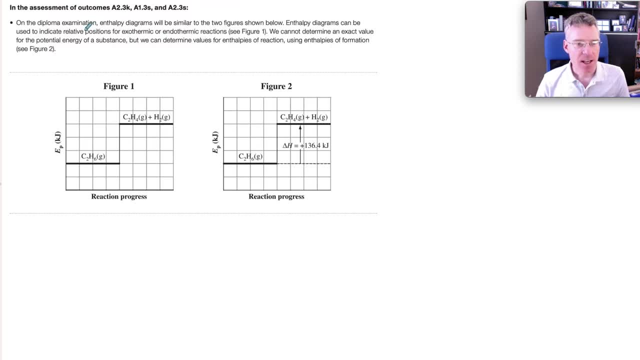 open versus closed and water vapor being a product or reactant. it's been in the bulletin twice. it's an outcome. make sure you know it. they just give an example of some of the chemical potential energy diagrams. even though you've learned about activation energies and barriers, you might see. 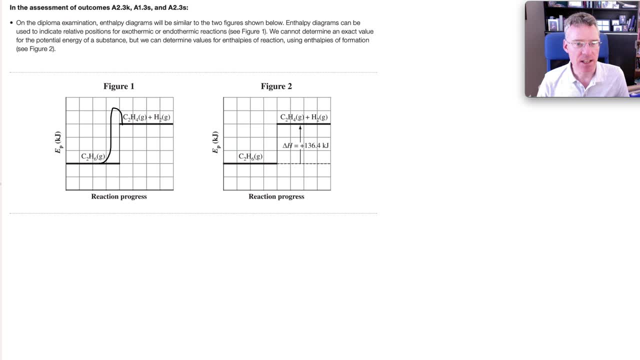 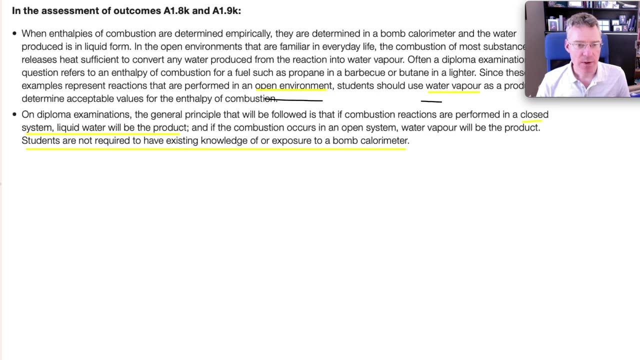 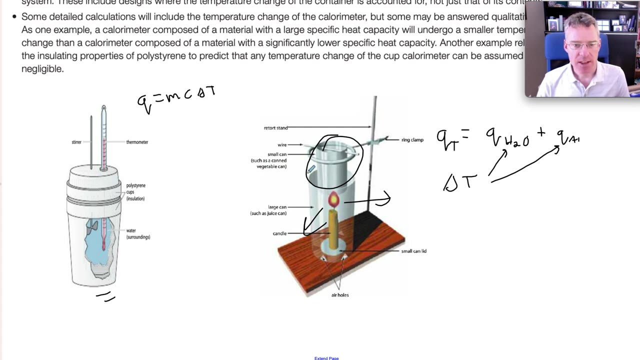 them without this barrier in front, and that's fine. that's something that that they'll do i mentioned a little bit ago. with the two designs of calorimeters- the styrofoam cup- efficiency is pretty close to 100. this setup can easily be 30 inefficient or 30 error. lots of heat can go out the side, depending on the heat shield you have. 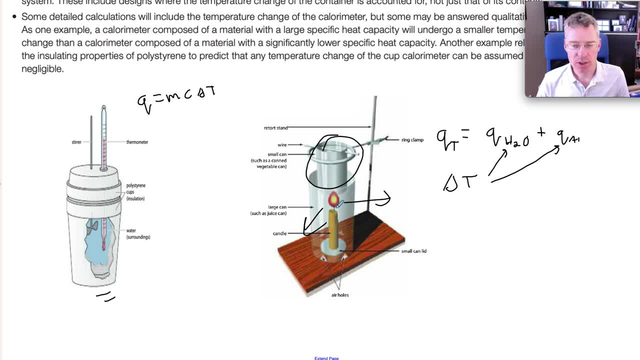 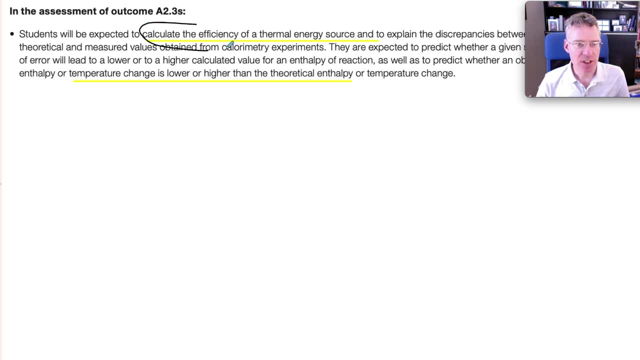 and the setup and how well you have your heat source or your your combustion reaction close to the can. you should be able to calculate an efficiency, so make sure you have done that. you're comparing the actual energy release to the theoretical value, and you should expect your efficiency to be. 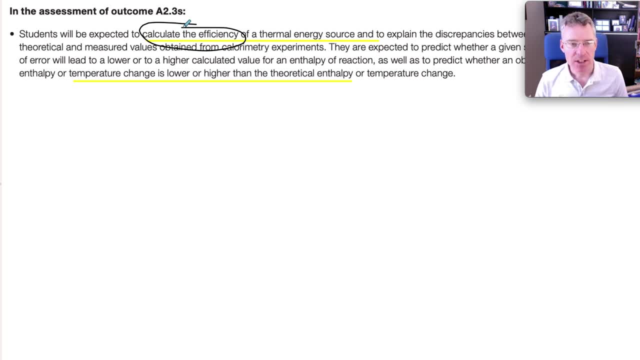 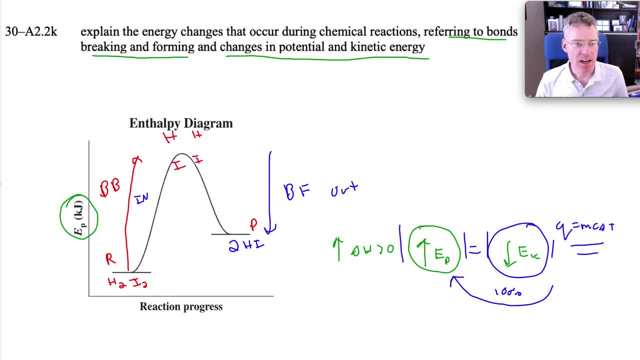 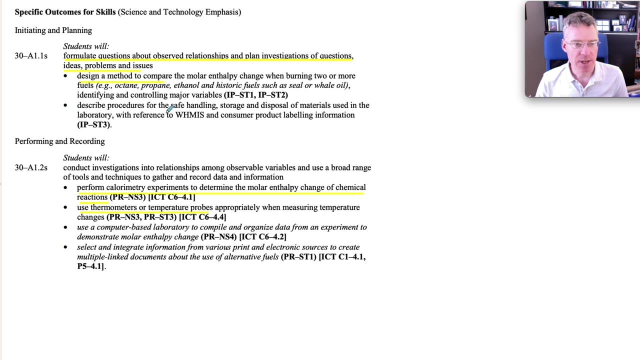 much less than a hundred. okay, this goes back to the that design type outcomes that i mentioned, and this is the most likely sort of application of the design outcomes that you might see on the diploma exam. your teacher would have had to have covered some of these planning and performing. 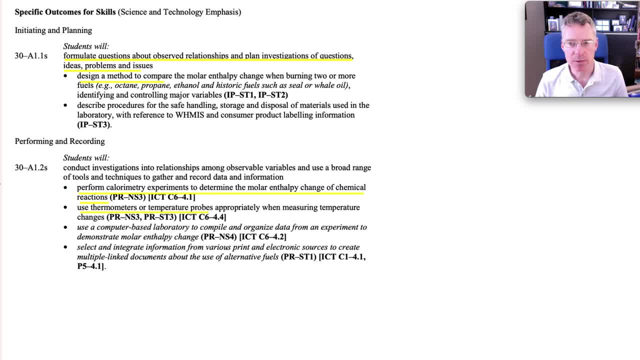 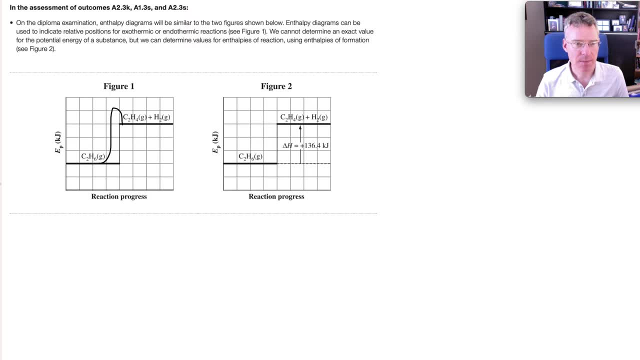 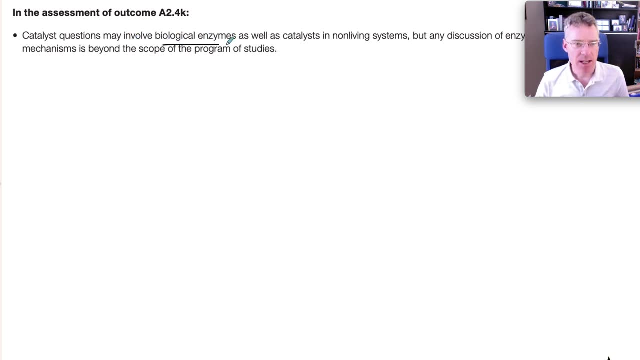 recording outcomes, but your diploma can kind of hit on it theoretically with with efficiency i mentioned. don't worry about the types of catalysts and enzymes. just any catalyst, regardless of the type, has the same effect. and and don't put time into studying different enzymes and how they work. 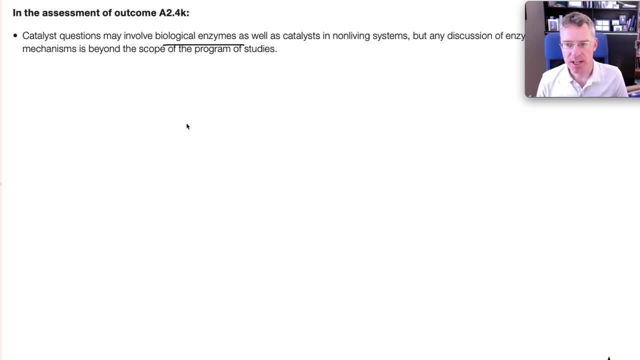 platinum versus biological ones. it doesn't matter enzymes or enzymes for the sake of of chemistry. 30. about tuning Customer Experience. download the application that you're getting into every day until next week, enthalpy with the diagrams or the term outside or the energy term inside. You might get more than